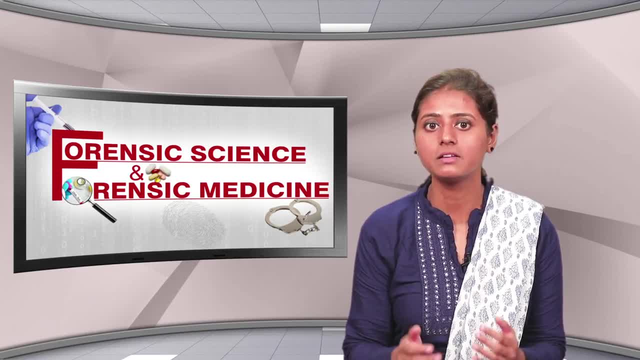 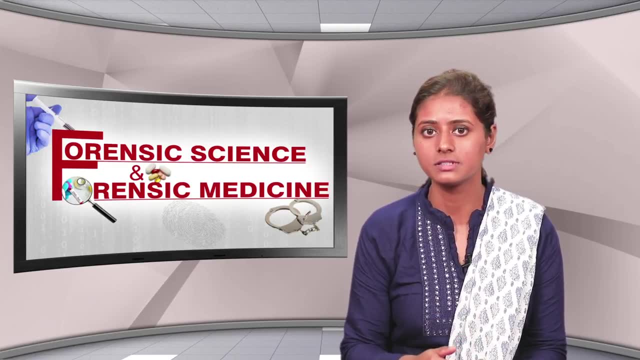 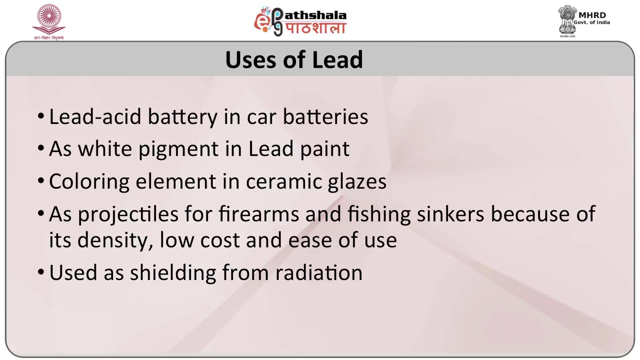 from ancient times. Lead pipes bearing the insignia of Roman emperors used as drains from the baths are still in service. Lead sticks were used as pencils, but not replaced by graphites. Uses of lead include lead acid batteries in car batteries as white pigments. 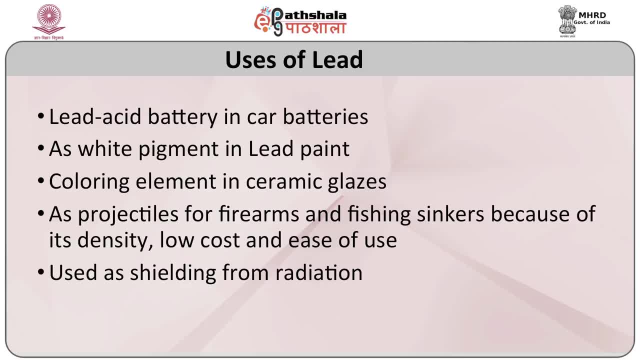 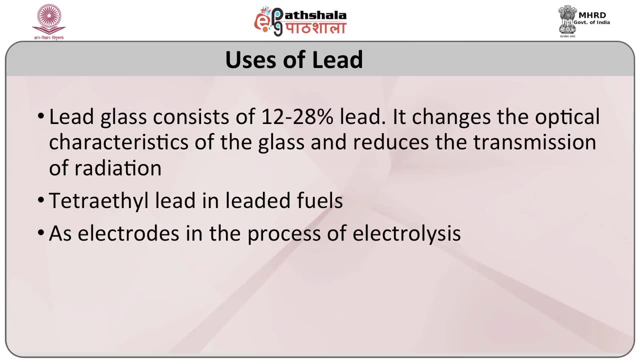 in lead paints, colouring elements in ceramic glazes as projectiles for firearms and fishing sneakers Because of its density, low cost and ease of use. Used as shielding from radiation, Lead glasses consist of 12 to 28 percent lead. It changes the optical characteristics of 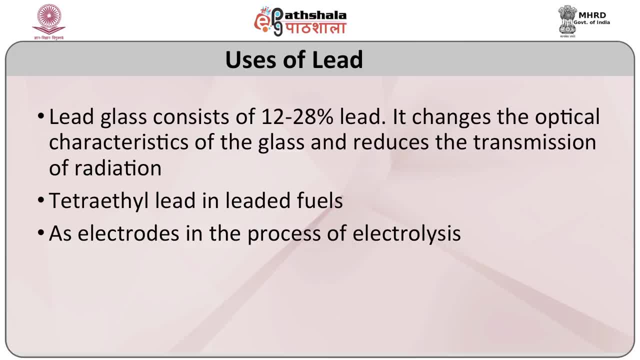 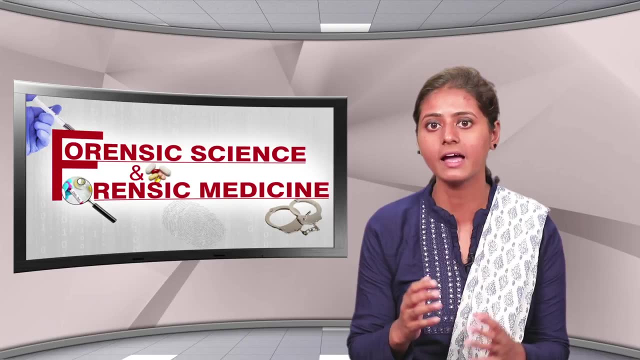 the glass and reduces the transmission of radiation. Tetraethylene lead in leaded fumes are used as electrodes in the process of electrolysis mechanism of action of lead, which involves one on a molecular level. lead inhibit or mimic the action of chemicals like calcium, which 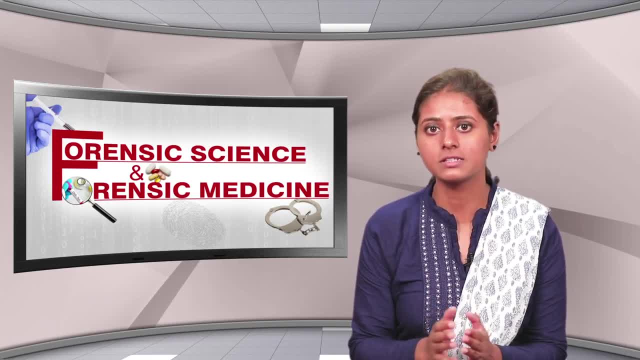 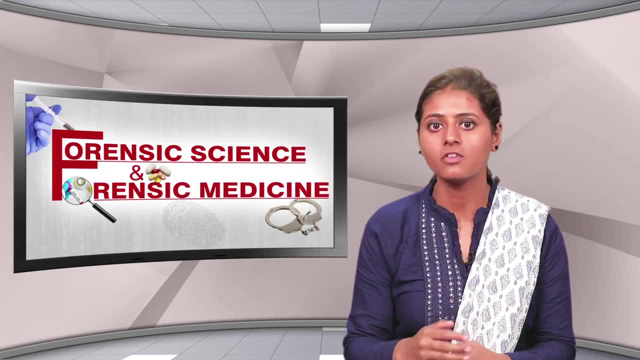 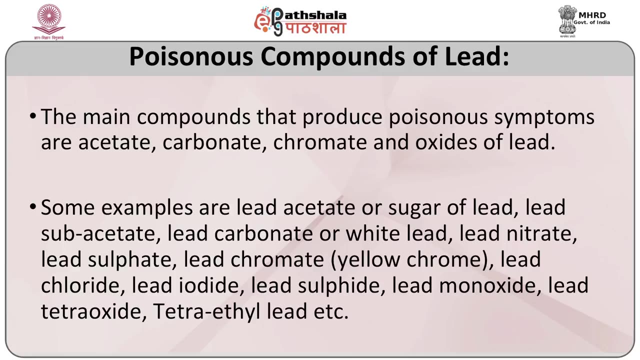 can affect calcium dependent or related processes and to interact with proteins, including those with sulphur, hydrolyzed amine, phosphate and carboxyl groups. Poisonous compounds of lead. The main compounds that produce poisonous symptoms are acetate carbonate, chromate and. 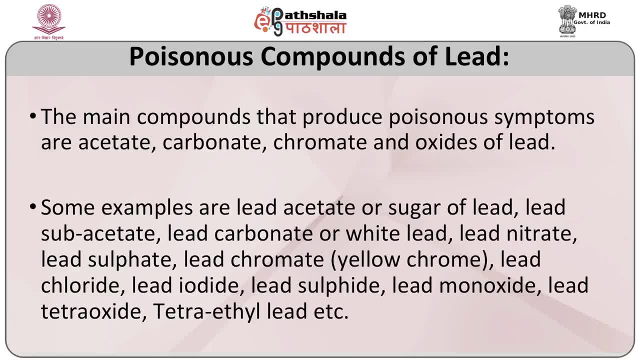 oxides of lead. Some examples are lead acetate or sugar of lead, lead subacetate, lead carbonate or white lead, lead nitrate, lead sulphate, lead chromate, which is also known as yellow chromate, lead chloride, lead iodide, lead sulphide, lead monoxide, lead tetraoxide. 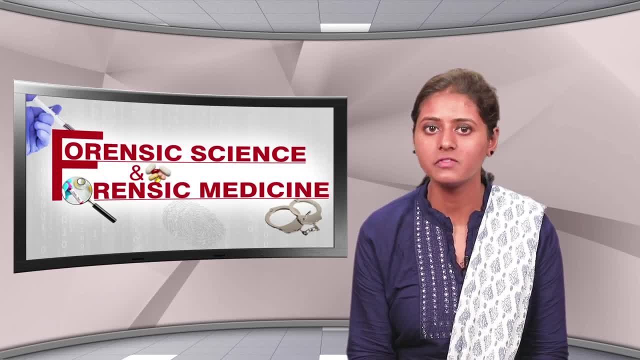 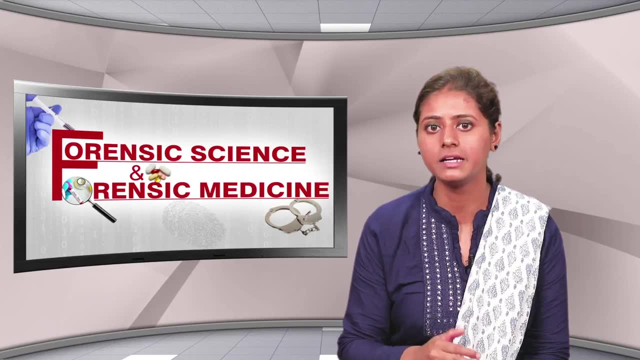 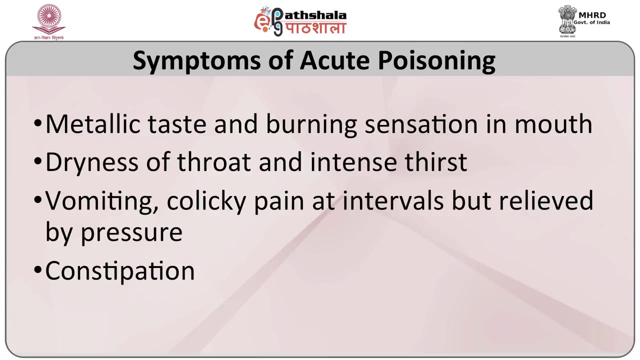 lead, ethyl lead, etc. We will discuss about acute poisoning. Acute poisoning occurs mainly due to lead acetate. The symptoms start immediately: Metallic taste and burning sensation in mouth, dryness of throat and intense thirst like vomiting cloaca pain at intervals, but relieved by pressure. 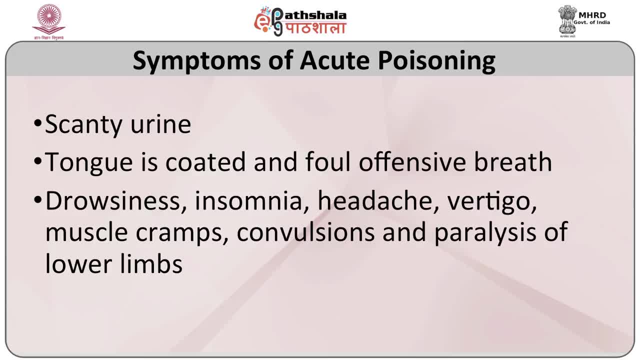 constipation, scanty urine, tongue is coated and foul offensive breath. drowsiness, insomnia, headache, vertigo, muscle cramps, convulsions. Acute poisoning occurs mainly due to lead acetate. The symptoms start immediately. Metallic taste. 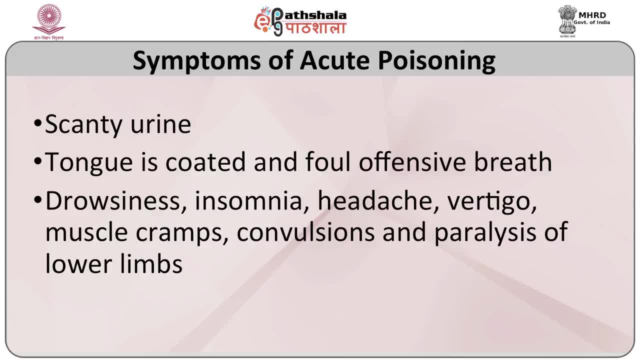 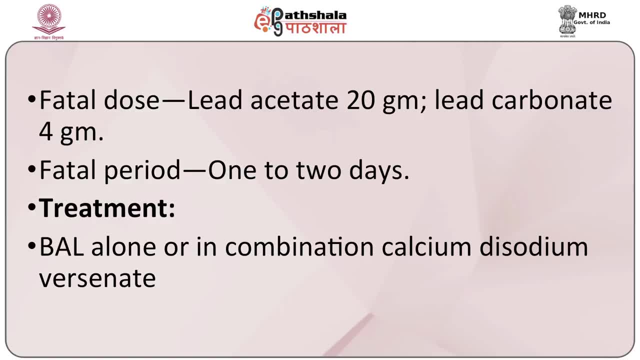 and burning sensation in mouth, dryness of throat and intense thirst, like vomiting cloaca pain at intervals but relieved by pressure, constipation, scanty urine, tongue is coated and foul offensive breath. drowsiness, insomnia and The fatal dose: Lead acetate 20 g. lead carbonate 4 g. Fatal period is about 1 to 2 days. 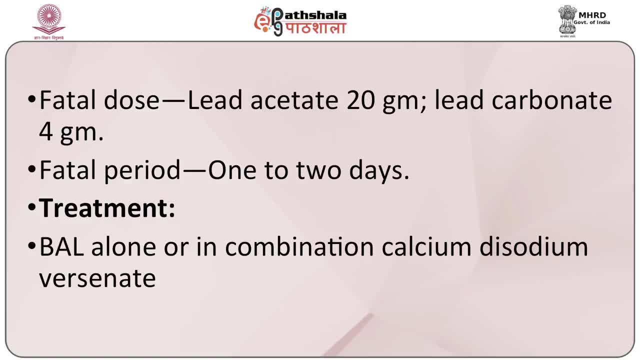 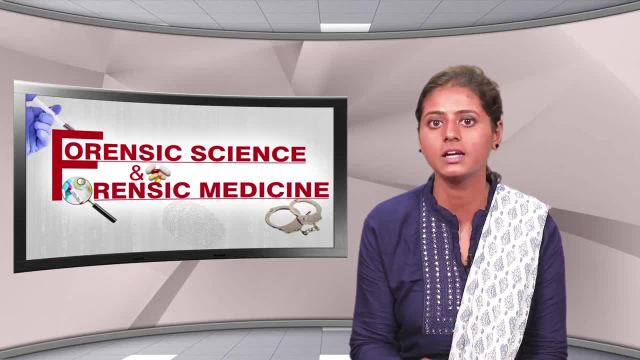 Treatment. The treatments for lead is val alone or in combination with calcium disodium, acinate or autopsy finding: Stomach, which may be from gastric mucosa, is congested, eroded and patchy in appearance with grayish white deposits. Large intestine may show blackish. 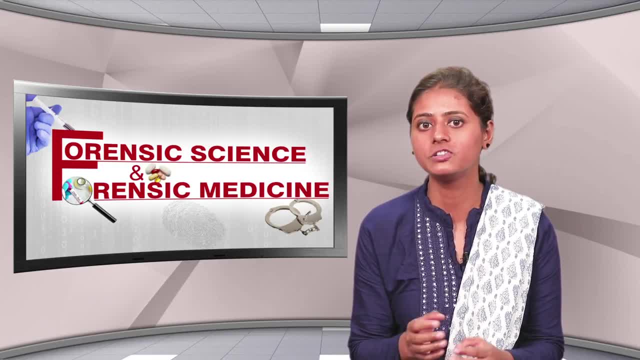 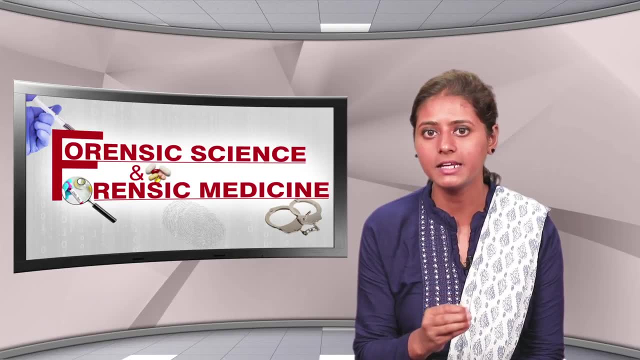 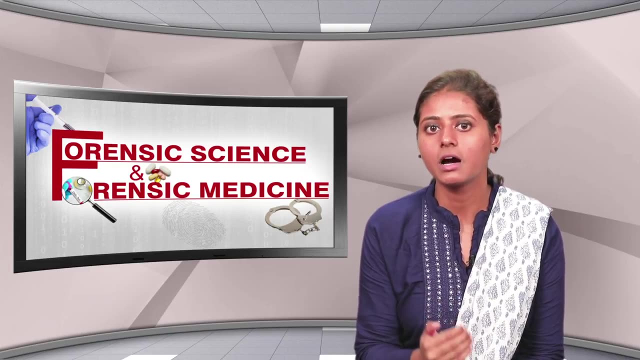 color fecal matter. evidences of renal tubular degeneration. chronic poisoning, which may also known as plumbation. Chronic poisoning occurs with a daily intake of 1 to 2 mg of lead. Sources of chronic lead poisoning: inhalation of lead fumes among persons working in factories. 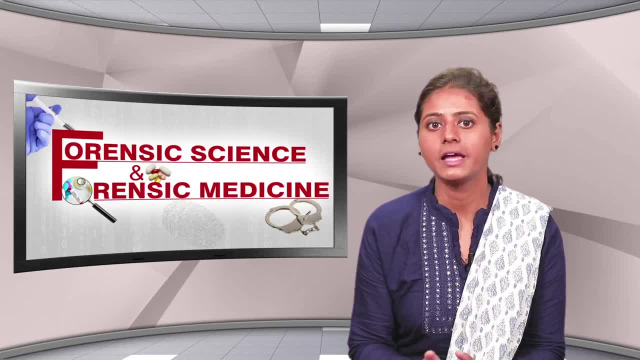 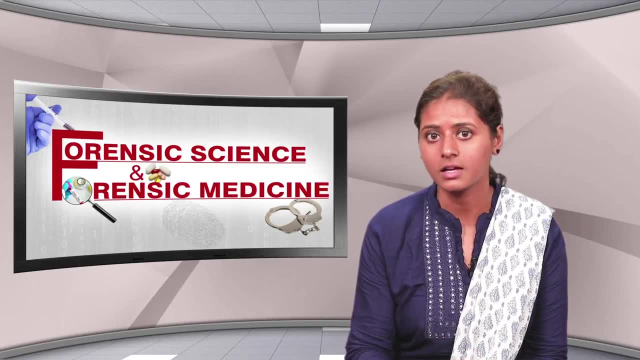 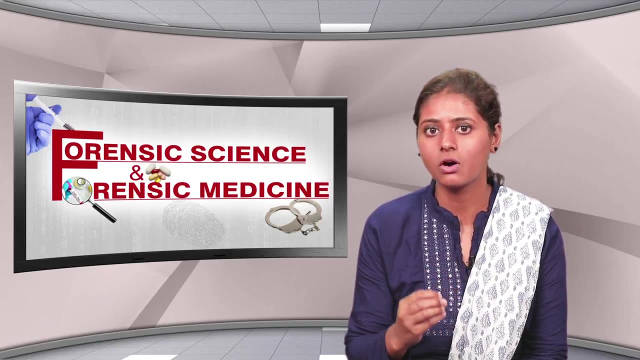 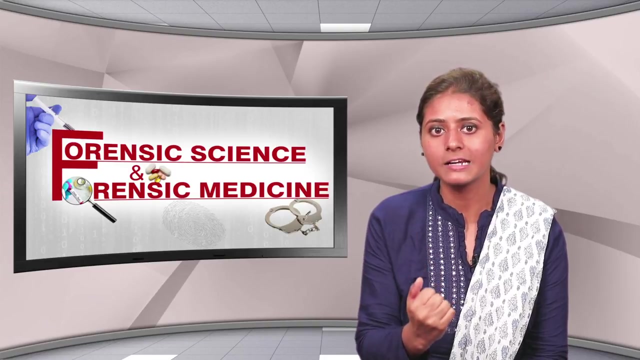 and industries such as painters, plumbers, enamel workers, glass boilers, electric lightworkers and lead smelters, etc. Eating tinned food contaminated with lead from use of ghee stored in brown or copper vessel may lead a line inside. with a tin Ghee become impregnated. 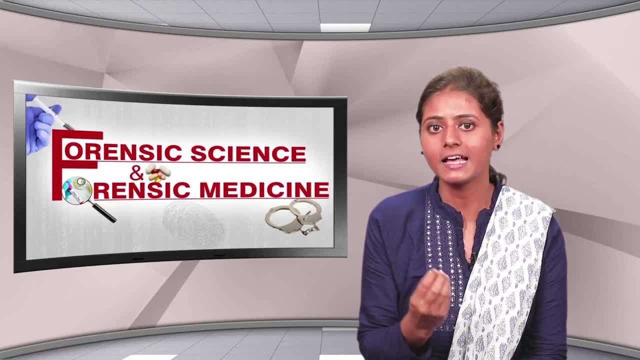 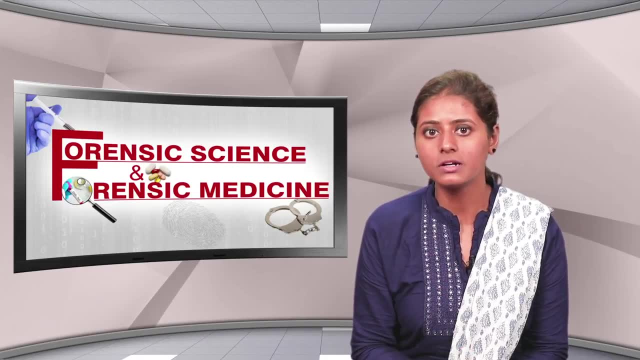 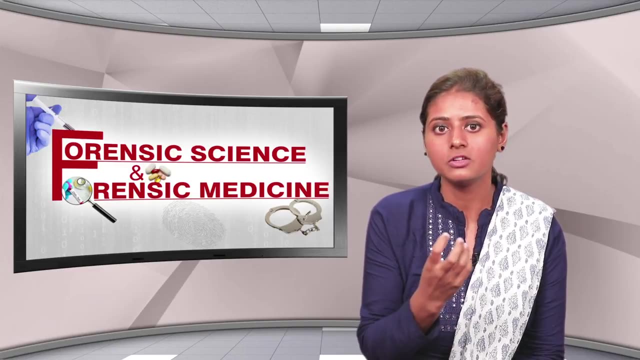 with a lead derived from tin that contains it as an impurity and forms a poisonous salt, which is also known as olate of lead. Food cooked in lead vessels may also cause absorbed of lead through skin. Hindu married- generally involve Hindu married females- apply vermilion. 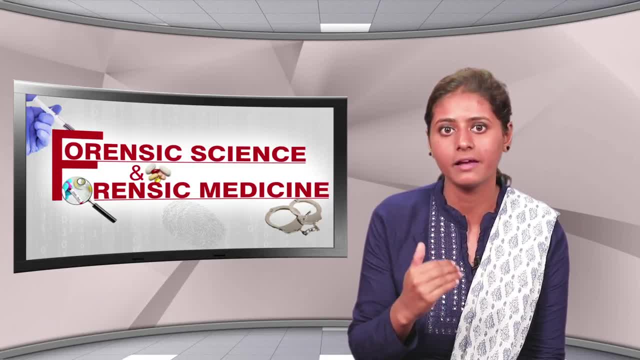 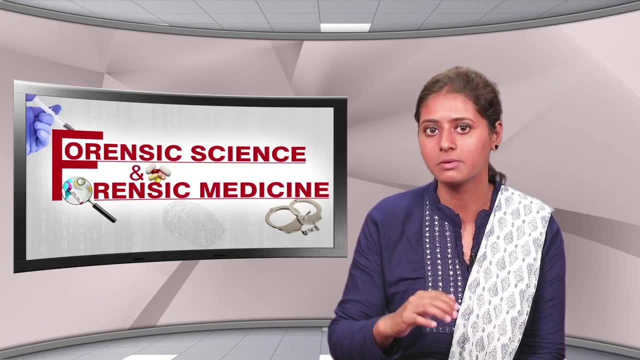 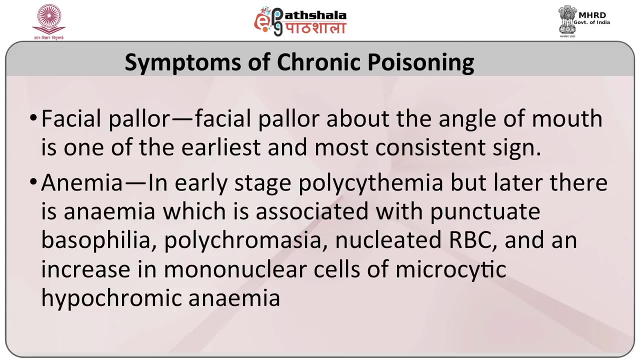 or which is known as sindoor, on the parting of scalp hair. Vermilion contains red lead mixed with red synthetic dye that can be absorbed through the scalp Signs and symptoms of the lead which is from facial paler, or facial paler about the angle of mouth is one of the 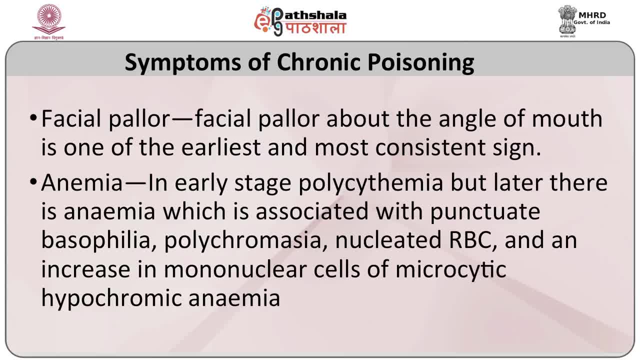 earliest and most consistent sign: Anemia in early stage polycythemia, but later there is anemia which is associated with punctuate basophilia, polychromatasia, nucleated RBC and an increase in mononuclear cells of microcytic hypochromic anemia. Lead line: a stippled blue. 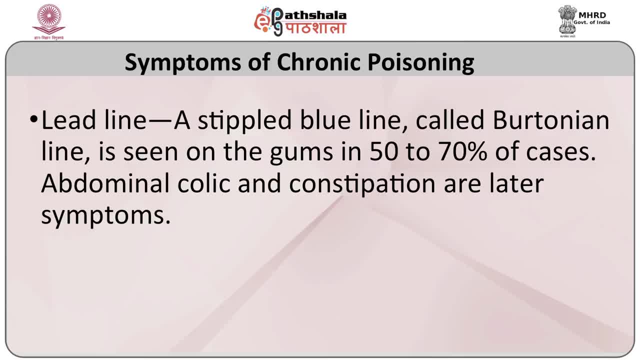 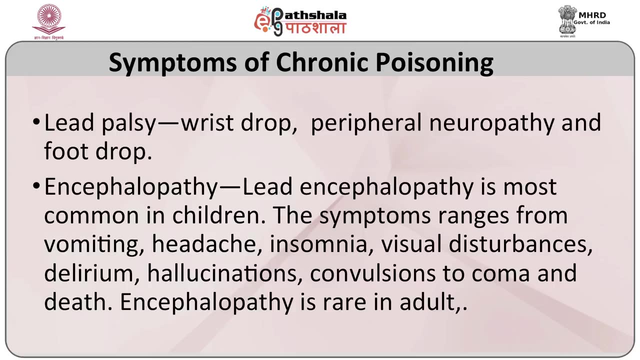 line called Bertoglialis. Bertoglialis line is seen on the gums In 50-70% of cases. abdominal tonic and constipation are later symptoms. Lead palsy, wrist drop, peripheral neuropathy and foot drop. Lead encyclopathy is most common in children. The symptoms ranges from vomiting, headache, 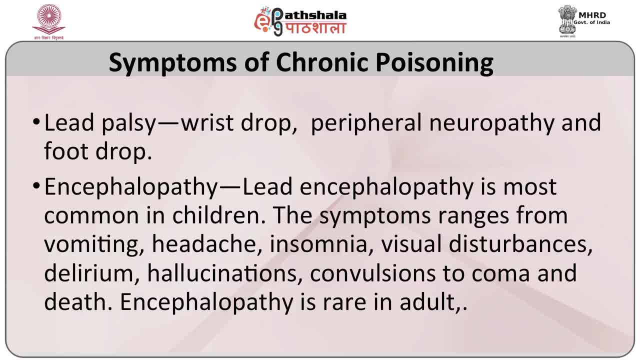 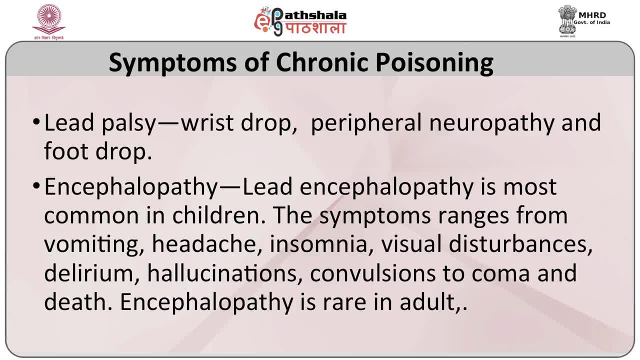 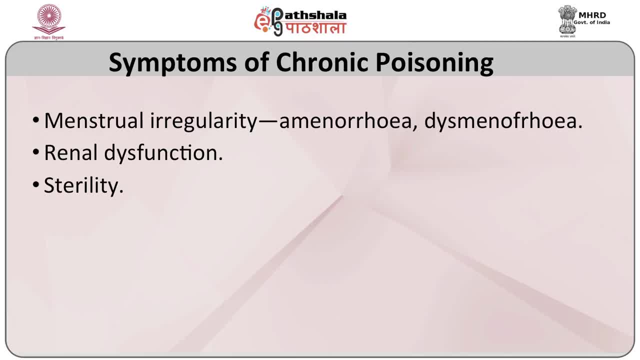 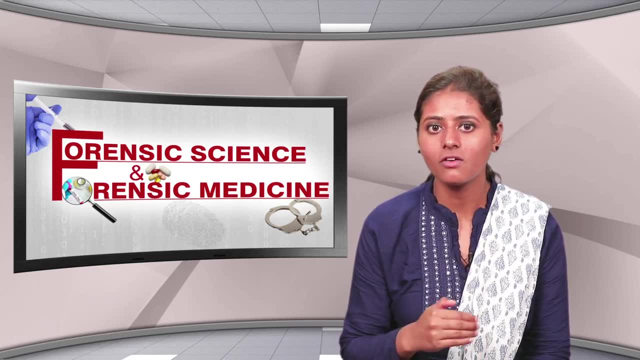 xylopathy are very common in adults: Menstruation irregularity, amnouria, dysmenorrhea, renal dysfunction, leptomy and sterility. Diagnosis of lead poisoning: In poisoning, the concentration of lead in blood is usually. between 0.1 to 0.6 mg per 100 ml. X-ray evidence of inoculation is very rare and the lead poisoning is only reported to be in the under 10 to 15 percent of cases. We have been working on a post-doctrine study to determine the coulombine castle bone and 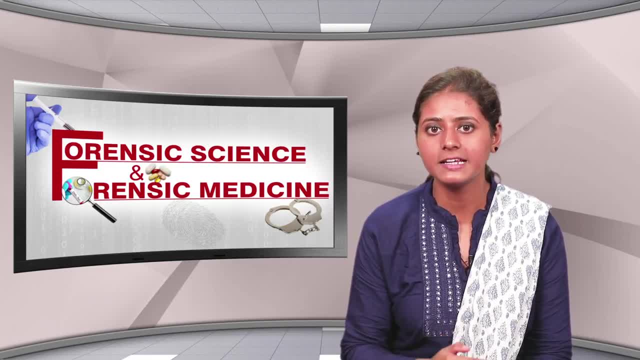 what is the risk of lead poisoning and how it affects the blood as well as the blood production in the blood. As a result, a number of live cells, brain cells and the blood. X-ray evidence of increased radial opaque bands of lines at the metaphyse of long bone. 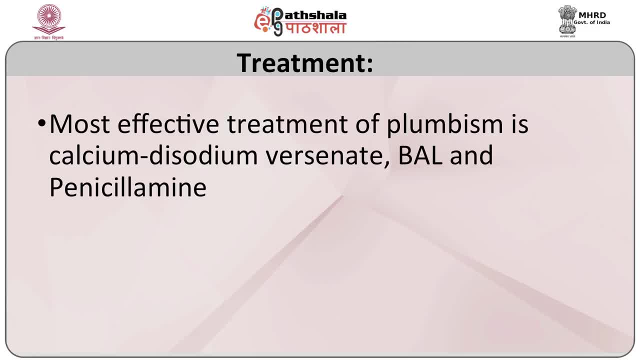 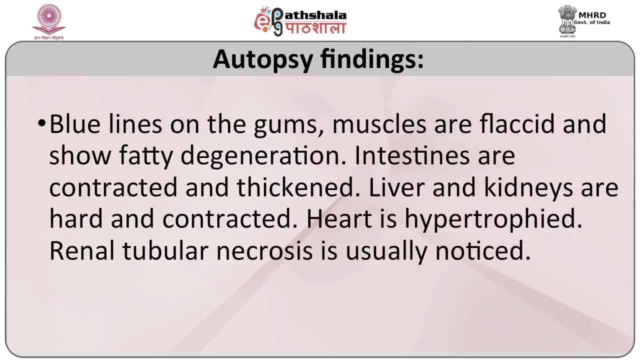 is seen in children's Treatments are most effective. treatment for the pulvism is calcium disodium versenate, or BAL, and the penicillamine and the autopsy findings, which includes blue lines on the gums. muscles are faceted and show fatty degeneration. 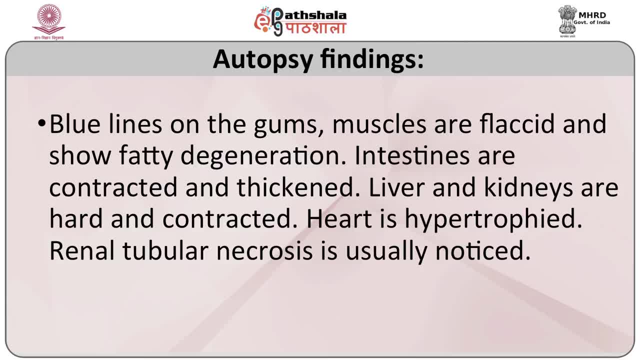 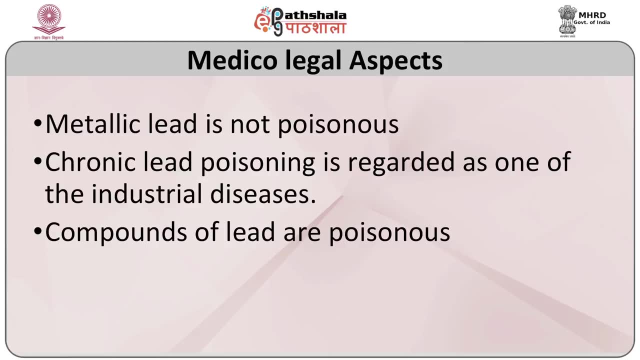 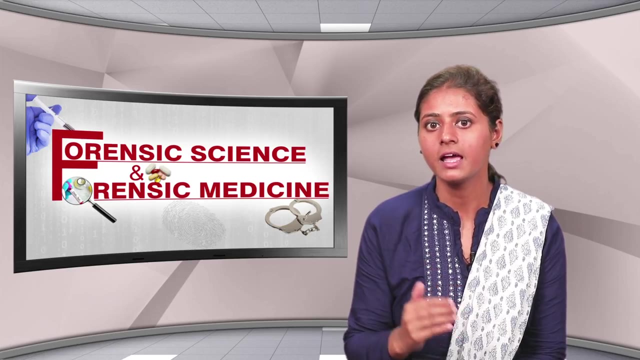 Intestine are contracted and thickened, liver kidney are hard and contracted, heart is hypertrophied. renal tubular necrosis is usually noticeable. The medical legal aspects of lead, the medical legal aspects which include metallic lead is not poisonous but when acted upon by secretion of the intestine and may lead as a poison. 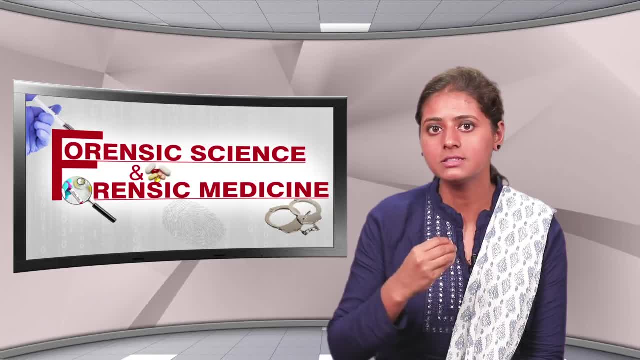 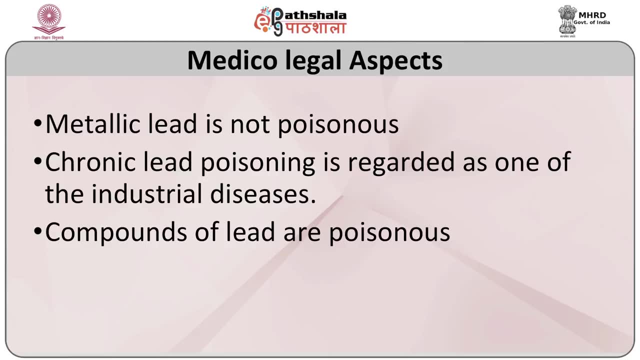 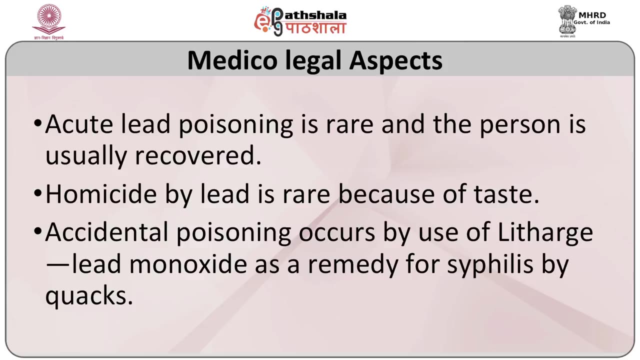 after being absorbed in the system, Calcium, as a salt. first, chronic lead poisoning is regarded as one of the industrial disease. second, compounds of lead are poisonous. third, acute lead poisoning is rare and the person is usually recovered. fifth, homicide by lead is rare because of taste. sixth, accidental 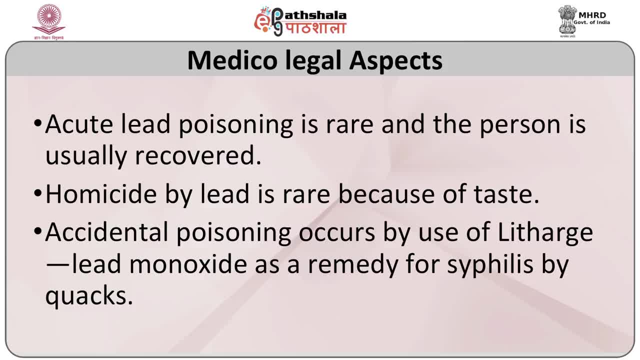 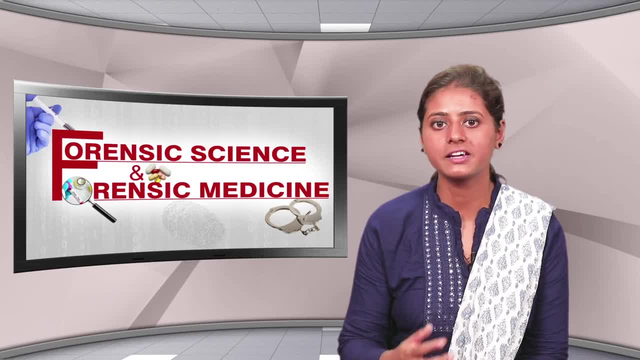 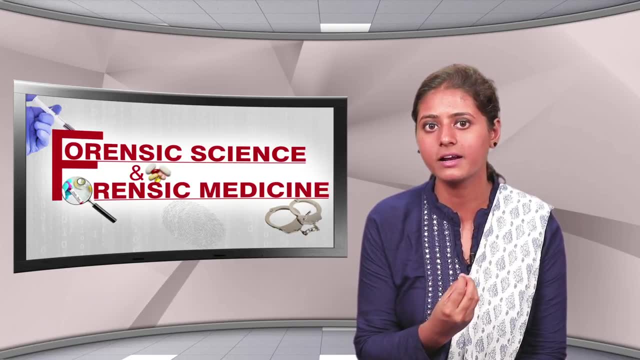 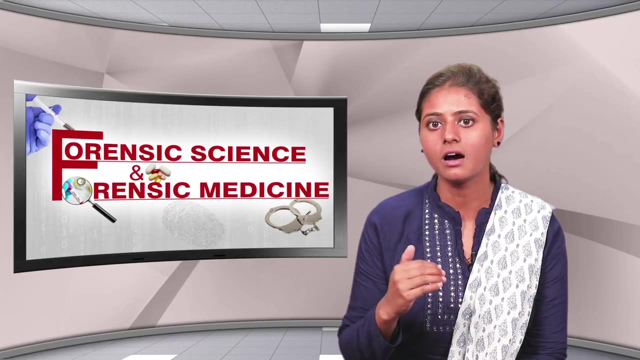 poisoning occurs by the use of lethargic lead monoxide. Seventh poisoning is called the cloroxyphysis by Quacks used as criminal abortifacients. the paste use on abortion stick contains red lead or red tetra oxide. Eighth cattle poison. red lead alone or when mixed with arsenic is used as cattle poisoning. 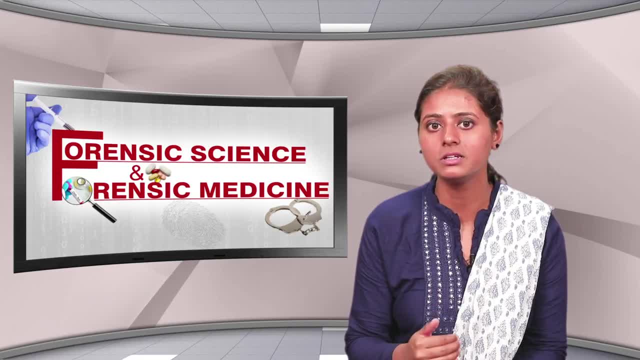 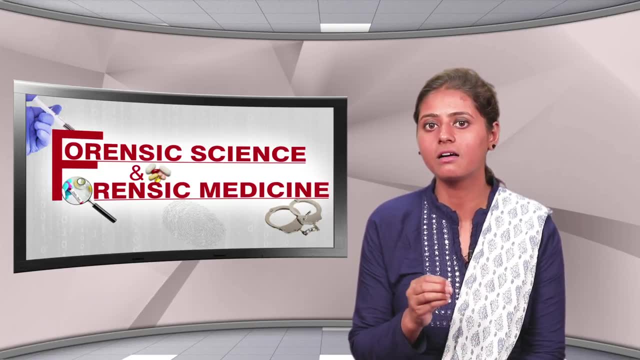 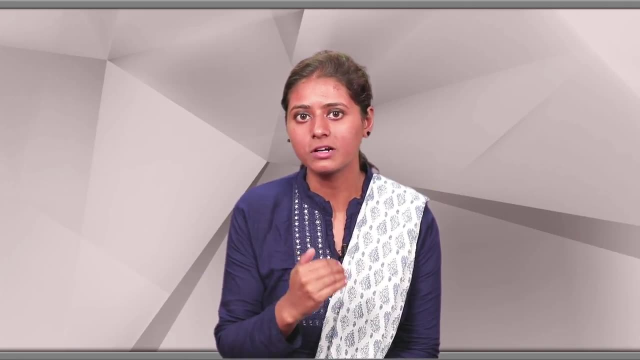 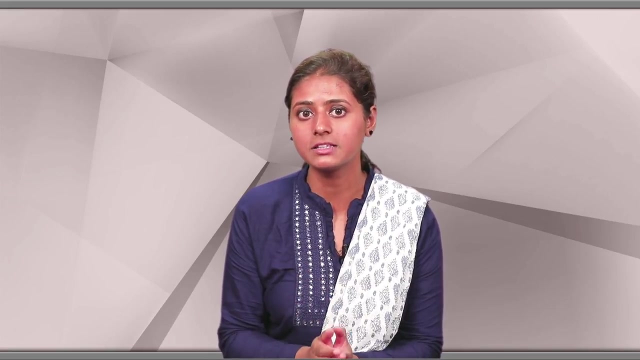 Tenth, lead is normally present in all human tissues deposited in the bones, nails, tooth and hairs, which is generally occur in the children's by eating Pika, old paint, plaster, feeding bottles made of glass contains lead. lead nipple shields, toys and street dirt cosmetics which may lead, like face powder, hair dyes used by the. 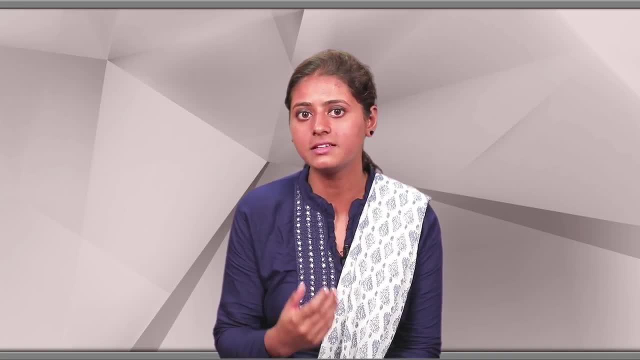 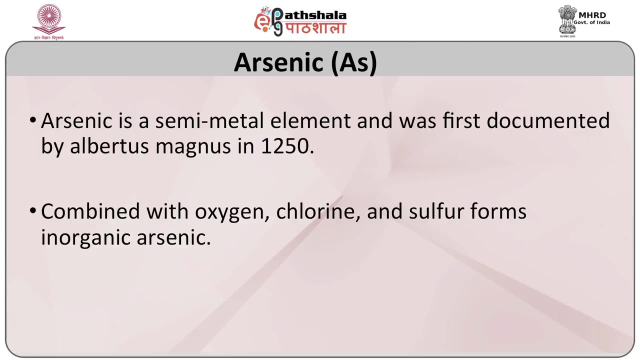 mothers secreted in the milk can cause accidental poisoning in the children's. now we will talk about arsenic. arsenic is a naturally occurring element and widely distributed in the earth's crust. when exposed to air, it combines with oxygen, which forms oxygen, or chlorine, and sulfur to form inorganic arsenic. 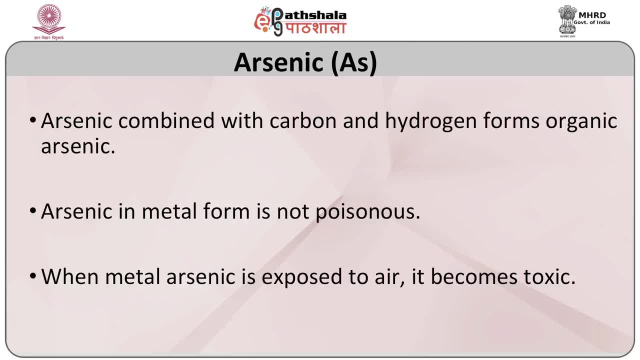 compounds. arsenic in animals and plants combines with carbon and hydrogen and form organic arsenic. inorganic arsenic are mainly used to preserve wood. arsenic is known to human since ancient times. the Greeks known it as early as 500 BC and hypocrites use it. 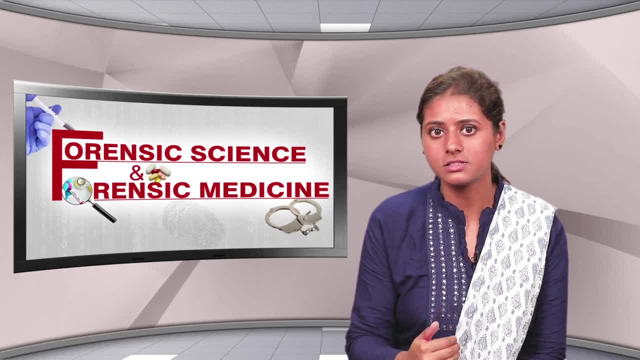 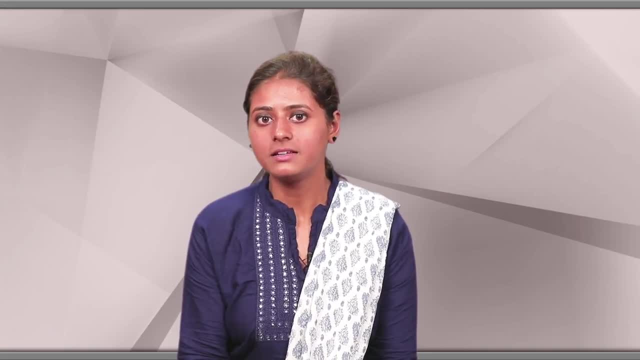 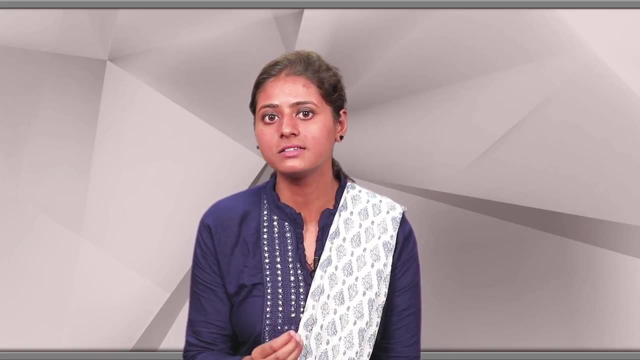 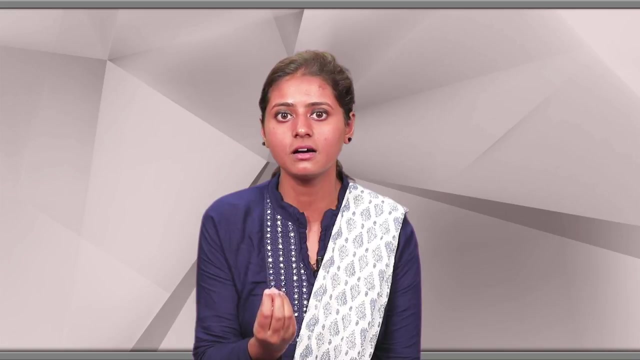 to cure body elements like ulcers, although there is no records of being used as a poison. this early and an 8th century Arab chemist, Javanese Jaber Ibn Hain, was the first to obtain white arsenic by heating real girl arsenic as has a very little smell or taste, so it is a undetectable by the 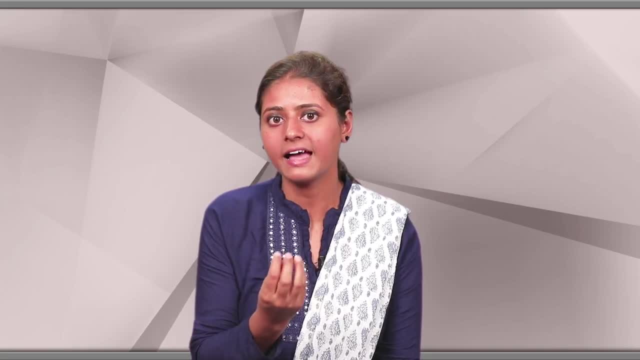 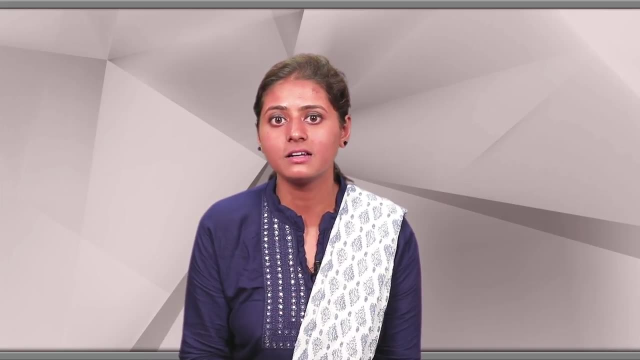 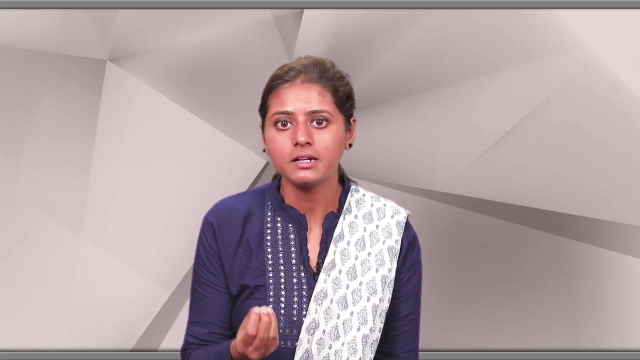 victim properties of arsenic, which includes the element which having number 33 in the periodic table and is considered as a heavy metal and environmental. arsenic is found in the form of sulfide complexes, real guard or payment and iron pirates. the metallic form is brittle and when heated it rapidly oxidizes to arsenic trioxide, which has a garlic order. the non mounting from is less reactive but dissolve when heated with a strong oxidizing agents and our colleagues arsenic gases, which is a use as h3 is another arsenic compound formed by the hydrolysis of metal. arsenis for a. 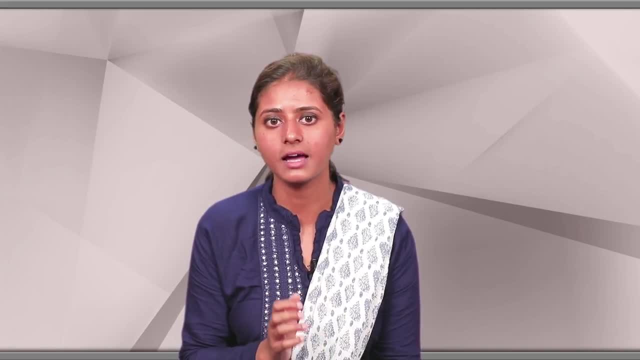 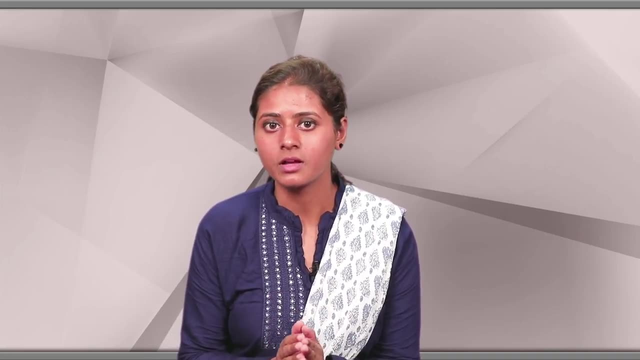 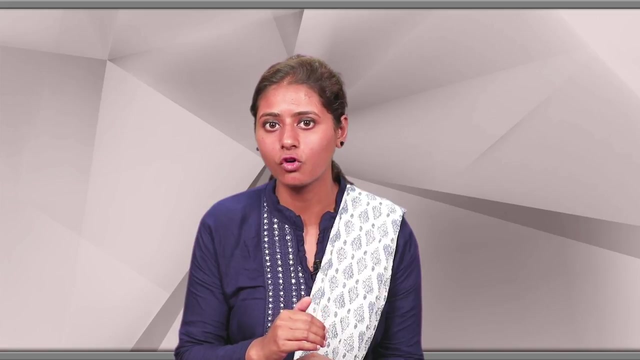 date and brasile iron produemphalule. let's loose our talk, but the key part of about those teachers in países aloj timber resources is found in the dieta ni and by the reduction of metals of arsenic compounds in acidic solutions. in elements form. arsenic is most poisonous as insoluble in water and can't be. 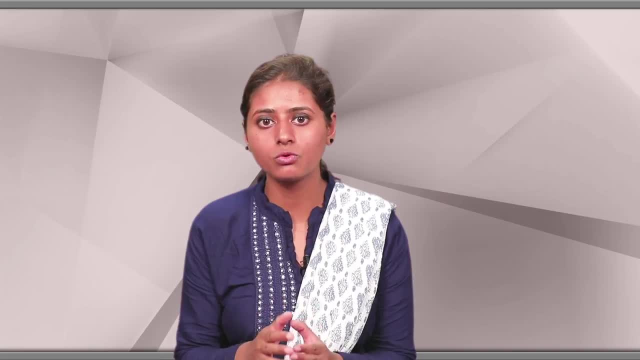 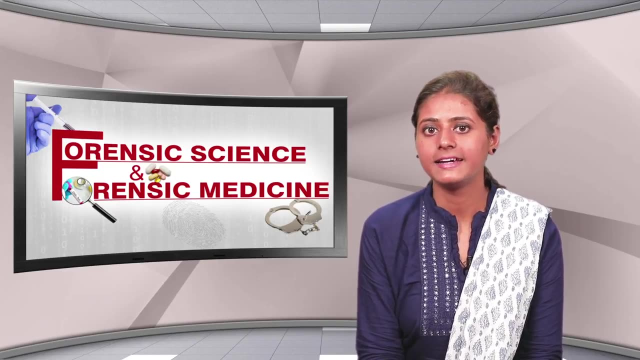 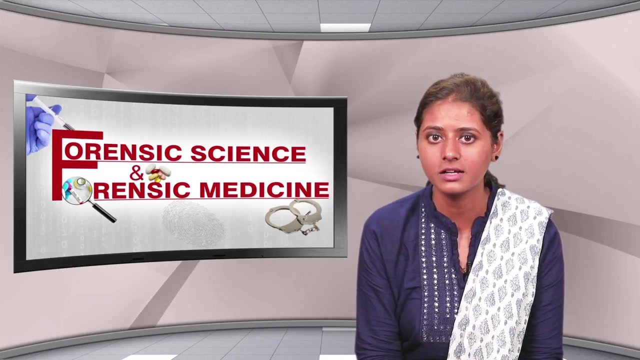 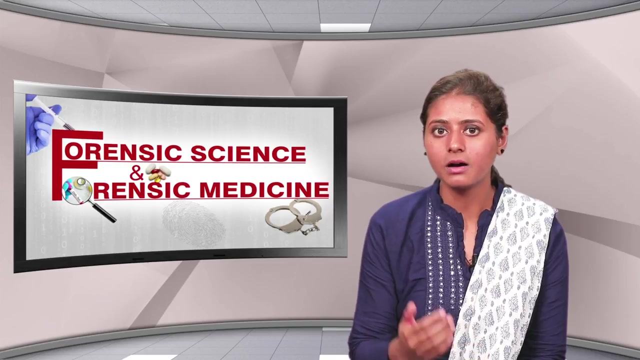 absorbed, but when it is oxidized by exposure to air it becomes poisonous. uses of arsenic: arsenic is widely used in calcium printing taxidermy, which is known as preparing mounting skin of animals, preparation of artificial flowers, wallpapers, preservation of timbers and skin against ants, mostly Hakeem's, and. 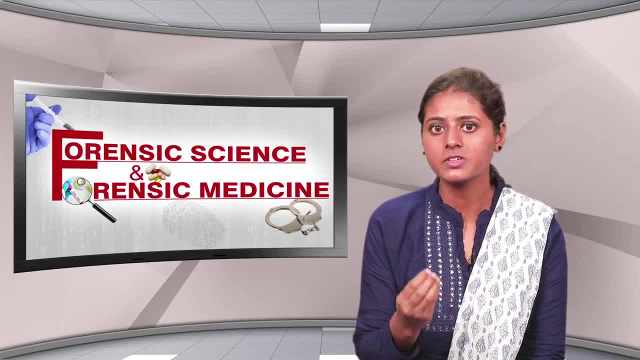 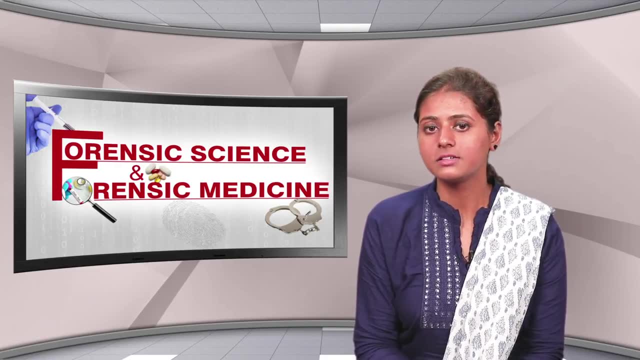 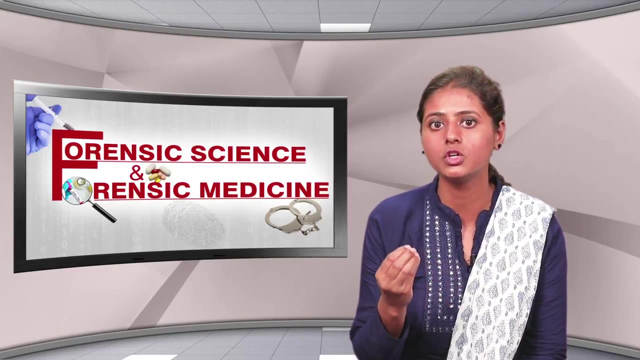 wads. use arsenic to treat rheumatism, skin disease, syphilis and impetus. natural sources of arsenic- the sources which include arsenic are: the average daily intake of arsenic in adults is about 0.5 % point five to zero point one mg. arsenic is found naturally in rocks and soil in concentration of less than one ppm. hot spring millions water drinking water supply. sea water contains about two to five milligram per liter in vegetables, fruits, grains, seafood, which is like fish, shellfish, crabs and no fish, etc. in industrial sources of arsenic, industrial process such as smelting of. 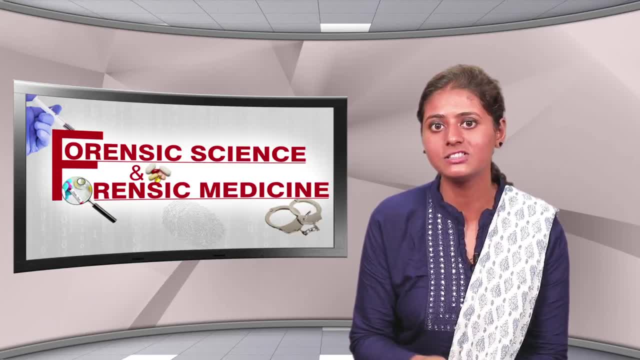 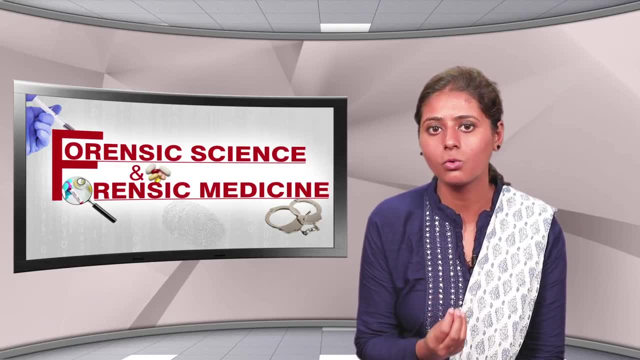 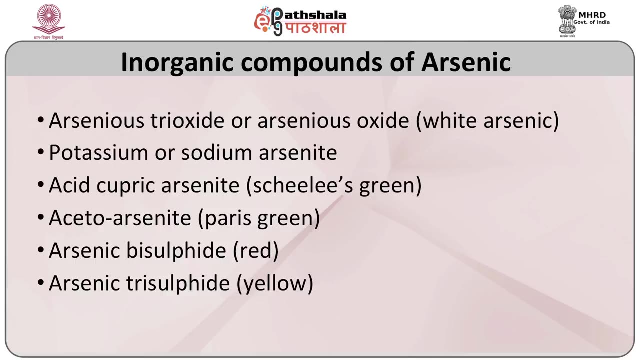 other metals. applications, which include arsenical, generation of power from coal, geothermal sources, which includes coal, and combustion of coal. the inorganic compounds, which include arsenic oxide or arsenic trioxide, which is a s2o3 copper sulfonite, which is seals screen, or Paris green red arsenic, or which is known as: 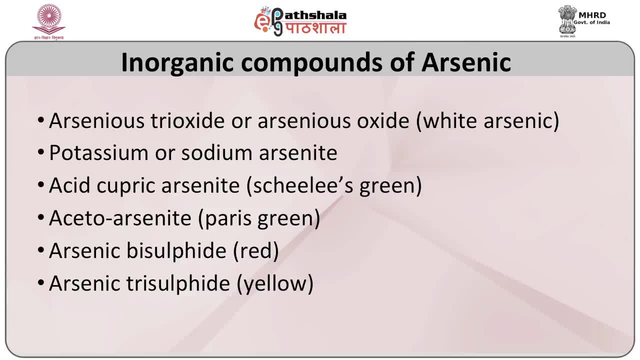 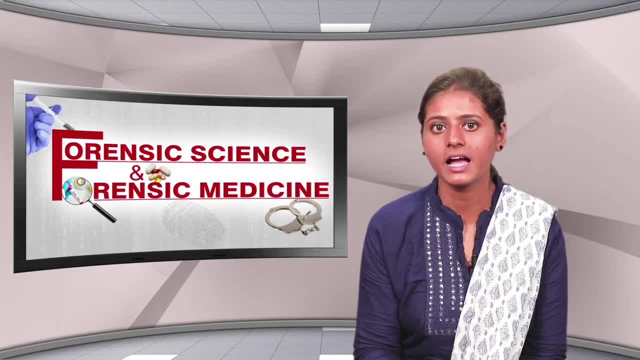 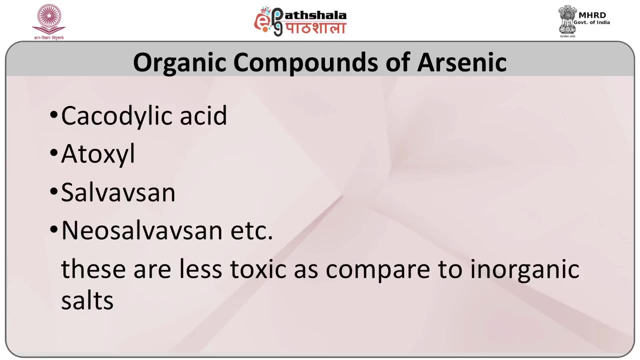 arsenic, arsenic disulfide or yellow arsenic, which is known as arsenic tri sulfide. arsine gas is. h3 is hemolytic and nephrotoxic organic chemicals. cocoa dialect acid, sodium. cocoa dilate a toxile salvation, new salvation. are there the mechanism? 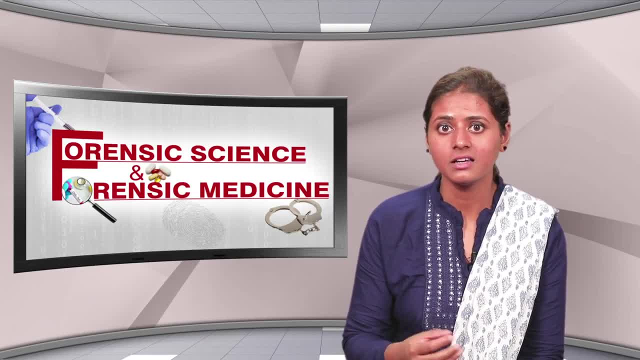 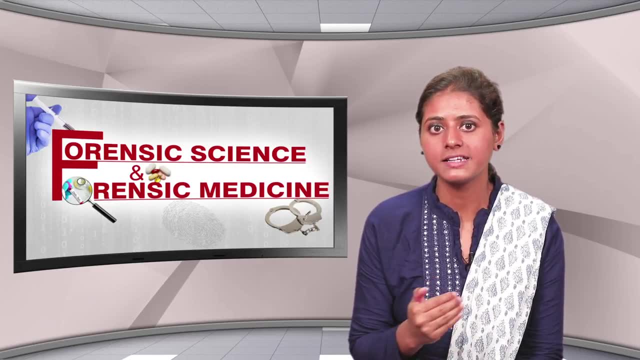 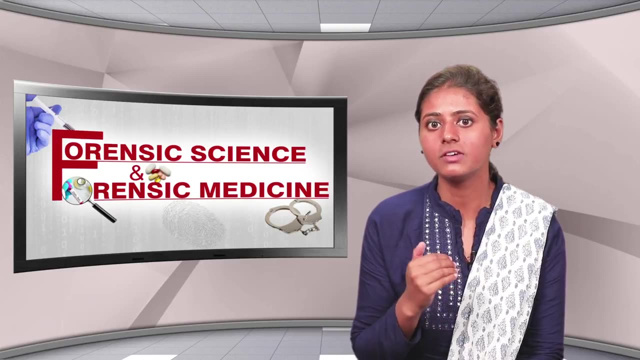 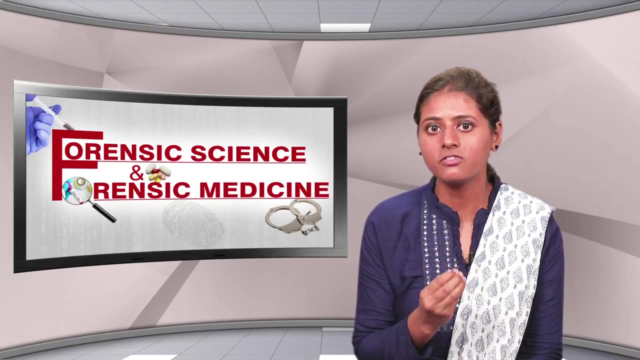 which includes the action of the lead arsenic. the mechanism of toxicity of all arsenic compound is the same. once in the tissue, arsenic exerts its toxic efforts through several mechanism, such as first include reversible combination with sulfur hydride groups, reacts with a stage group and tissue proteins it interfere with. 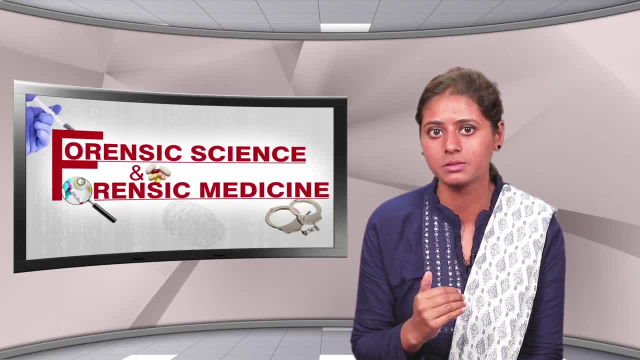 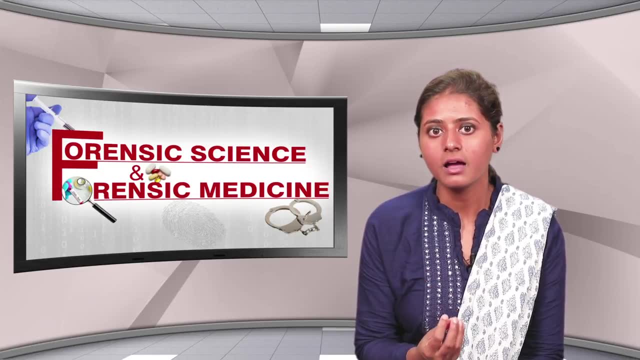 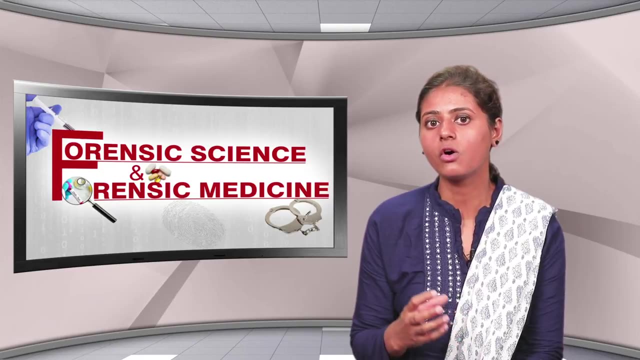 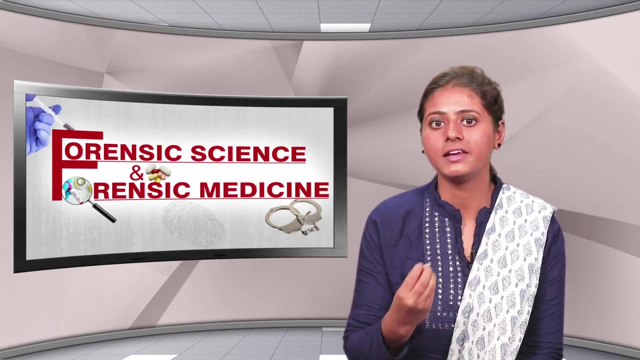 the enzyme system essential for the cellular metabolism, which dilates capillary fatty degeneration in the liver, hyponemia and hemorrhages in the intestine, or which may be renal tubular necrosis. the acute poisoning of arsenic are, which includes the results from the oral indition inhalation: arsenic gas rubbing. 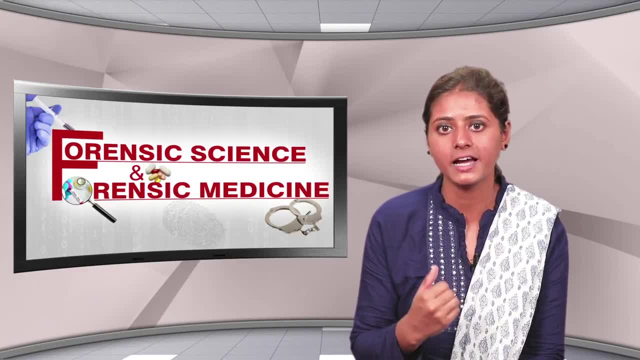 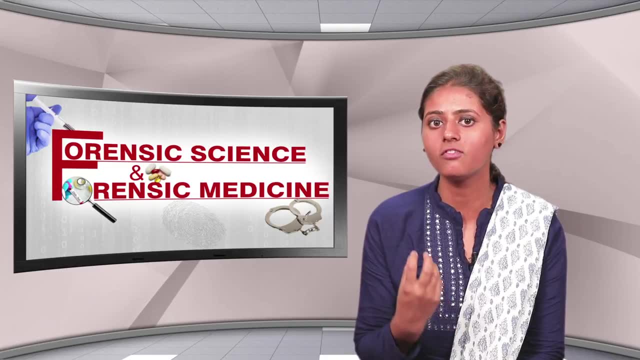 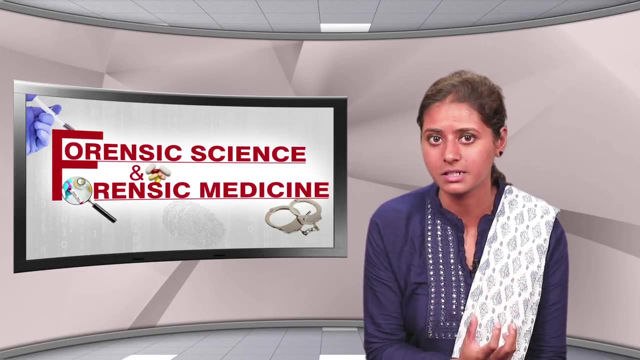 into the skin, introduction to rectum or vagina. arsenic poisoning is usually the result of accidental or suicidal indition of insecticides, which is also known as Paris green, that is, copper, arsenic, arsenic or calcium or lead arsenic. pesticide containing arsenic is fresh. his source of poisoning. the toxic symptoms of acute arsenic poisoning also depends upon the individual susceptibility or the fatal dose, which includes. the fatal dose of arsenic trioxide is 180 milligram, but the dose depends on type of the compound ingested, its physical form and the in her. inherent tolerance of the patient. now we will discuss about the fatal dose. the fatal dose of arsenic trioxide is 180 milligram, but the dose depends on type of the compound ingested, its physical form and the inherent tolerance of the patient to arsenic. the fatal periods is the for arsenic poisoning is about 12 to. 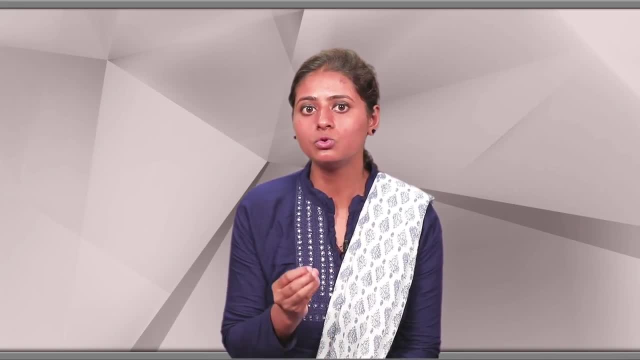 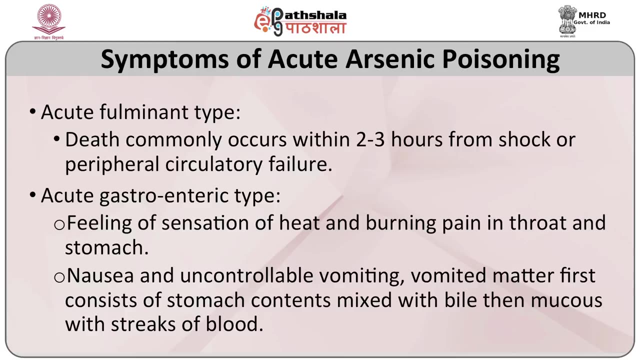 48 hours, but can be fatal even within 2 to 3 hours. the science and science model signs and symptoms are: the feminine type: excessive large doses of arsenic can cause death and then three hours from shocks. second, the gastroenteric type: this is a acute poisoning resembling bacterial food poisoning or cholera. this 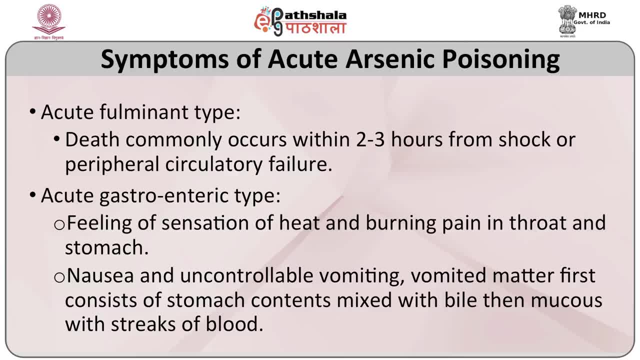 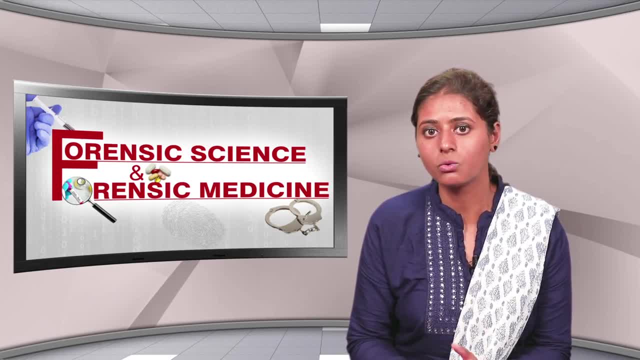 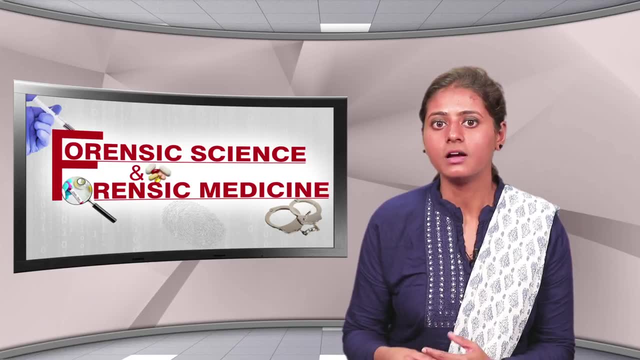 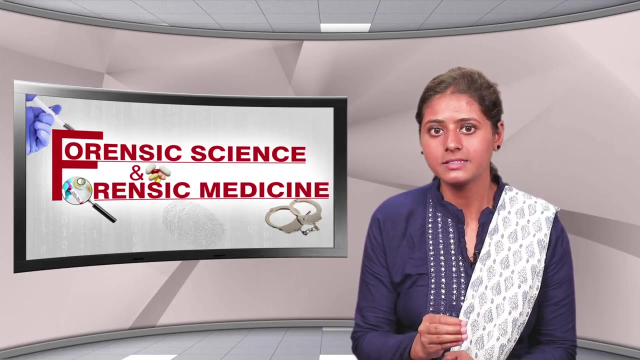 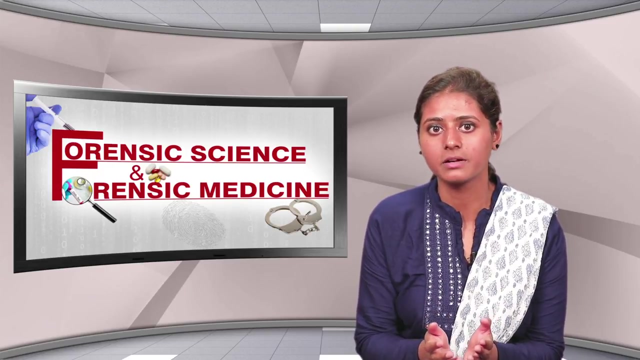 tool are expelled frequently and involuntary, dark colored, stinking and stained with the blood, but later becomes colorless, odorless and water resembling rice water. stools of cholera, dehydration with muscular cramps, synopsis or feeble pulses, syncope, coma or exhaustion, conversion or general, maybe paralysis can be happen and death, skin eruption are common. the symptoms which are caused by death are caused by the loss of blood as well as the dead skin. by this are necrotic forms, tenderness of the muscles, delirium, coma and death. fatal doses of this, which are 0.1 to 0.2 gram or 100 to 200 milligram fatal. 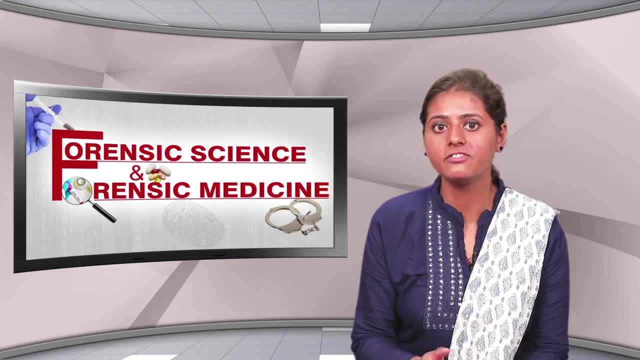 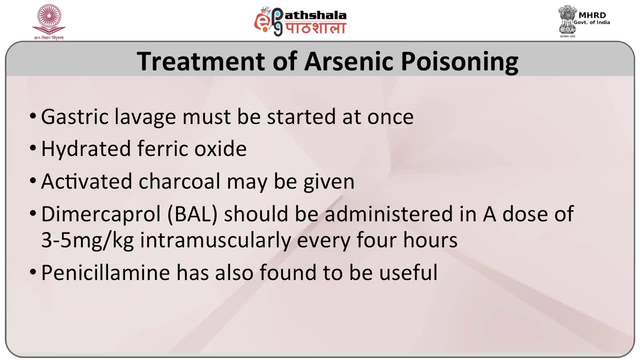 period, which include 1 to 2 days, or differences between arsenic poisoning and cholera. let's just talk about the treatment. freshly prepared precipitates, hydrate, ferric oxide, or which is also known as arsenic antidote, and arsenic poison ball is used as an antidote- or maybe calcium dis sodium, arsenate or and. 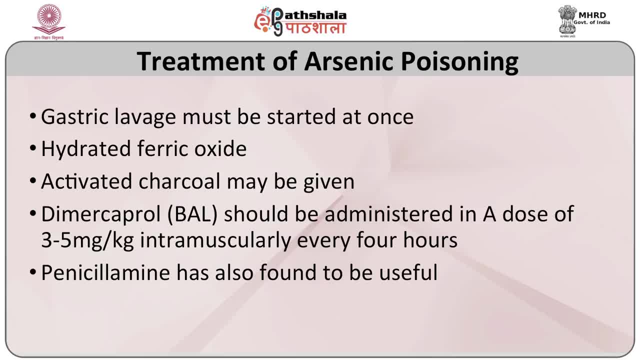 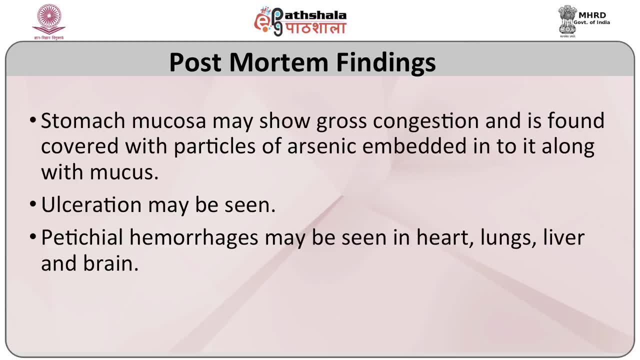 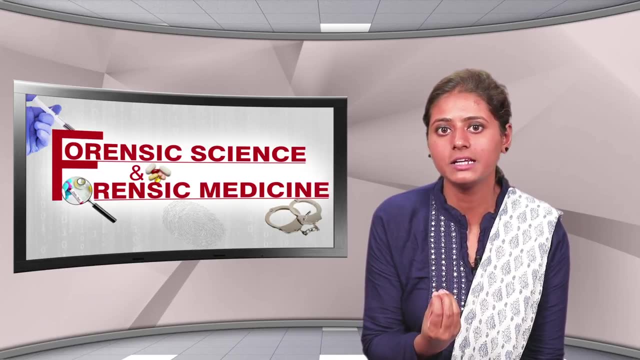 pencili 9 are also helpful: the post-mortem appearance- maybe read velvet, velvety appearance- of the stomach mucosa or the chronic poisoning which is include the first, which is known as CNS, polymerase, neurotic and optic neuritis. the second skin, finally, which is molted brown. 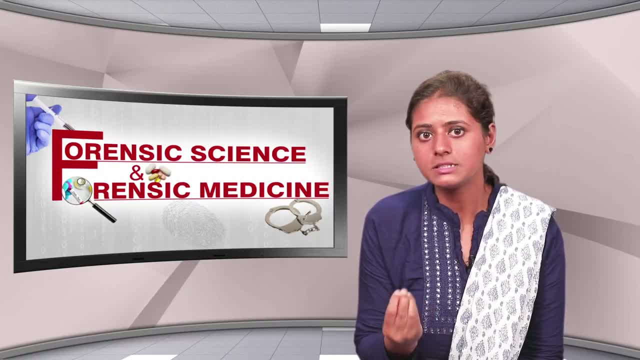 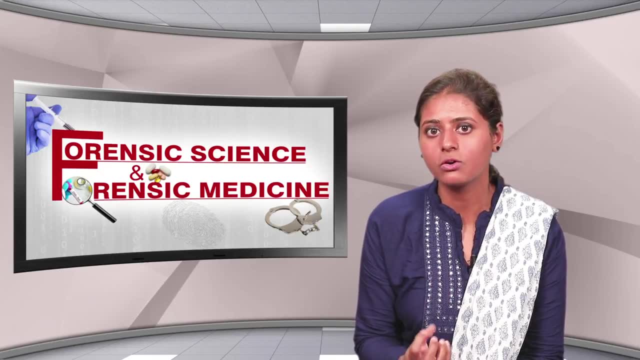 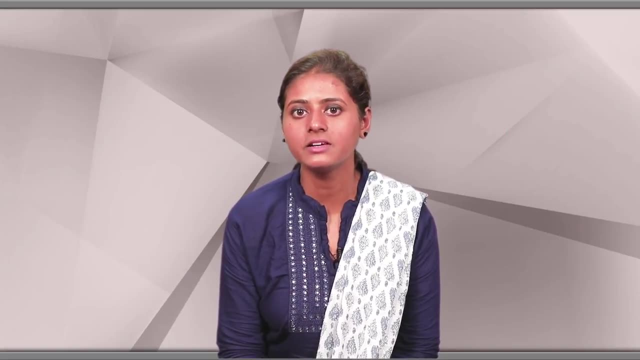 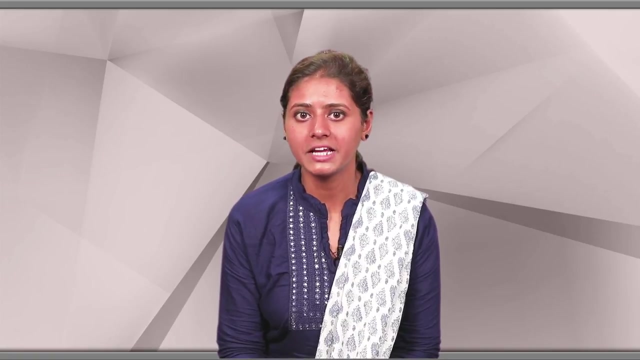 changes, mostly on the temples, eyelids and neck, which may be rain drop appearance. a chronic ice arsenic poisoning causes basal cell carcinoma, liver cirrhosis. there may be a rash resembling fading measles, rashes, hyper cataracts and hyperpigmentation of the part and source with the irregular. 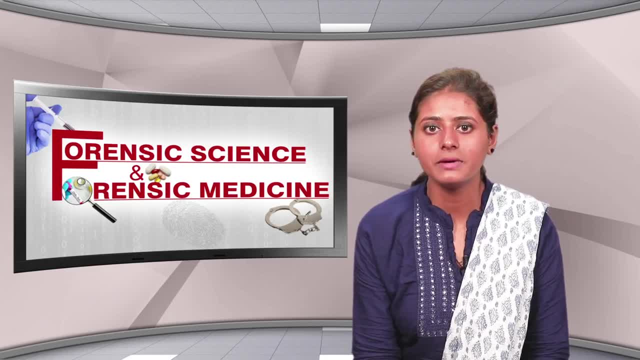 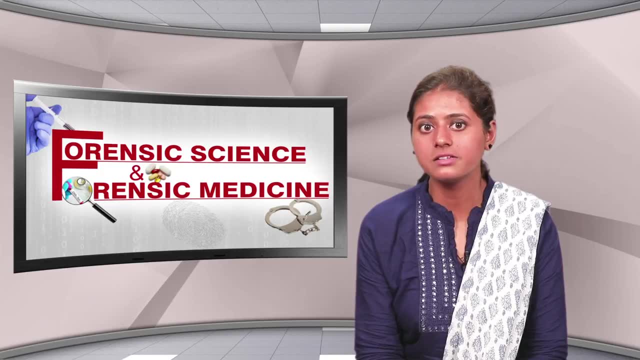 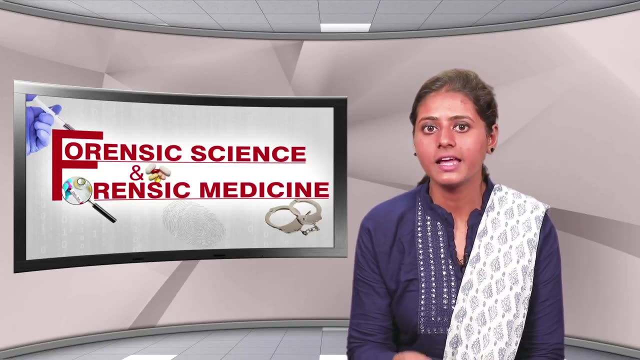 thickening of the nails is seen. next, development of bands of opacity in the fingernails are called Eldridge mess line. as you know, phagocytes are people who take arsenic daily as tonic or as an aphrodisiac, and they acquire a tolerance of it about 0.3 grams or more in one dose. 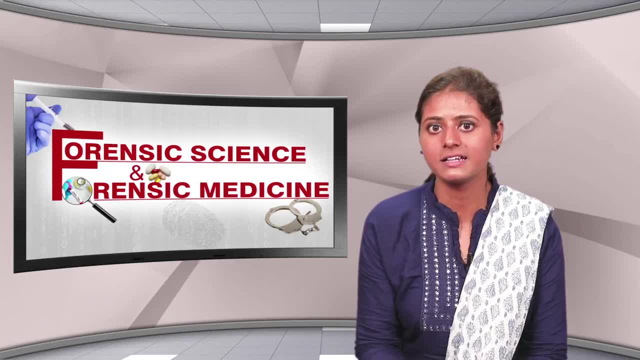 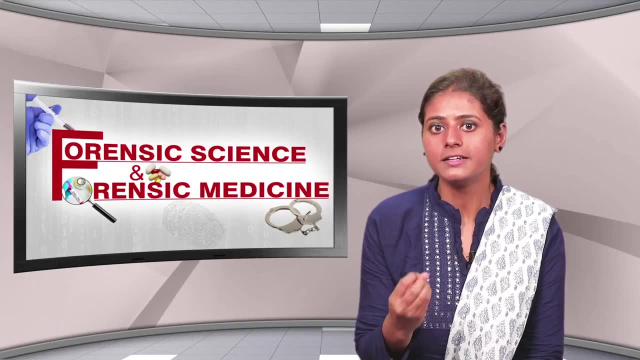 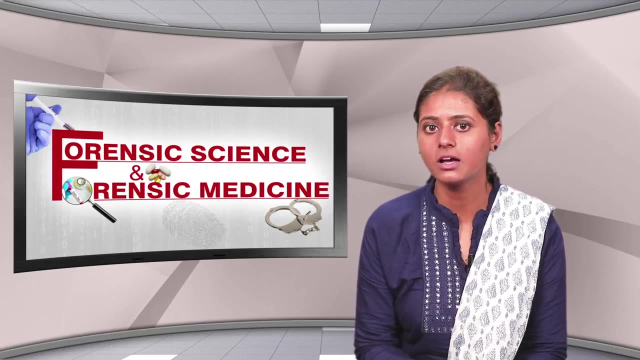 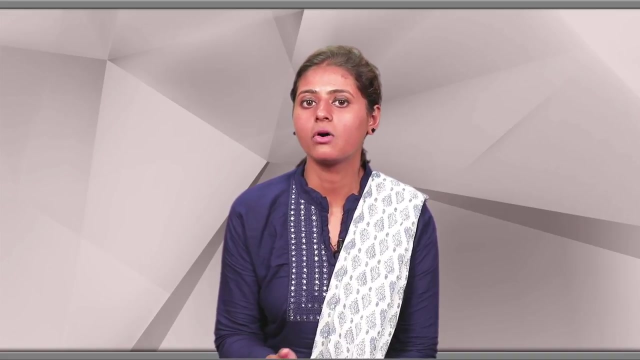 you can see the difference between arsenic and. arsenic is the most popular homicidal poison and it delays putrefaction. it can be detected in completely decomposed body. it can be found in bones, hairs and knees for a long time. it can be detected in charred bones and acid. it is sometimes used in abortion sticks tests. 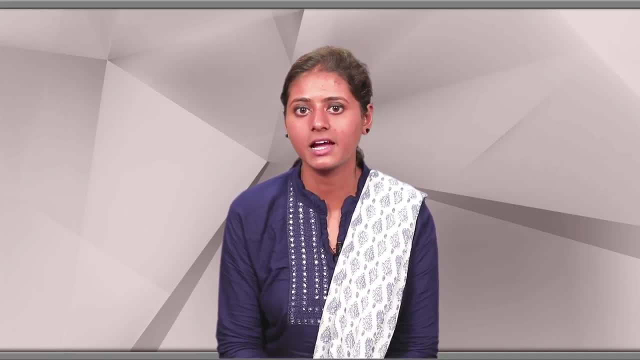 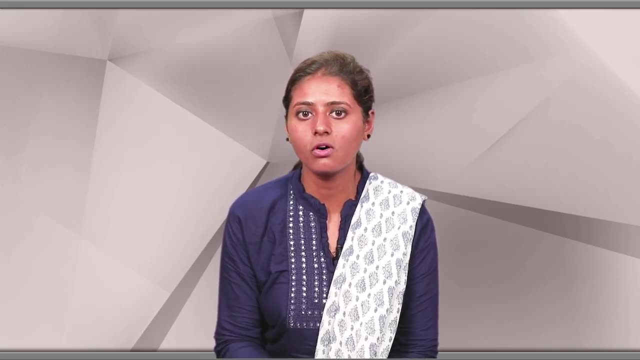 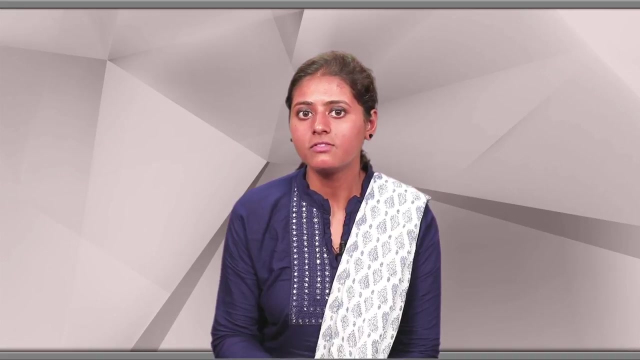 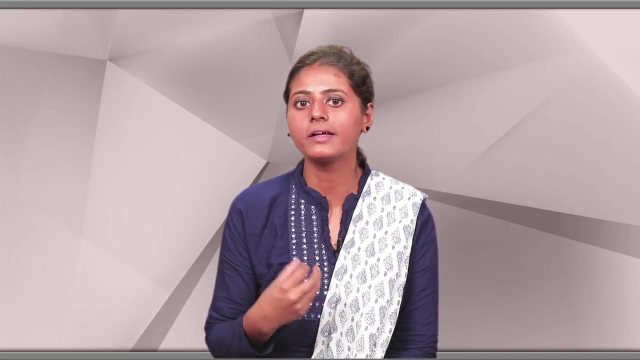 for the arsenic detection, which includes master's tests and wrenches tests. so we will now discuss about the mercury. the mercury combines with the almost all elements like chlorine, sulfur, oxygen, forming inorganic compounds or salts which are used well a powder or crystals. mercury can also combines with carbon to make organic mercury compounds, which is methylmercury is produced by microscopic organism in the form of perceberium and the water. Metallic mercury is dense liquid and vaporizes easily at room temperature. Metallic mercury is not absorbed into unbroken skin. However, it vaporizes even at room temperatures. 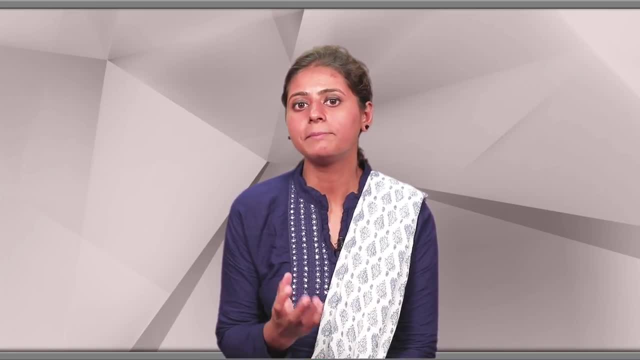 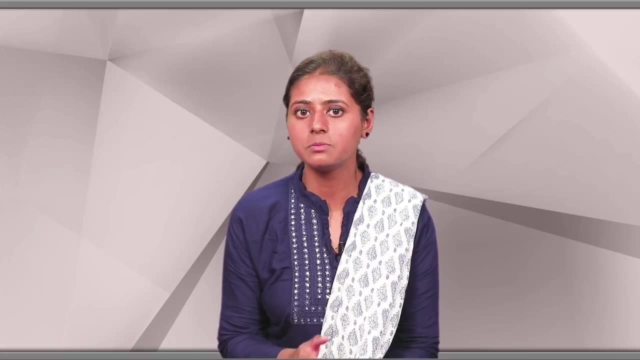 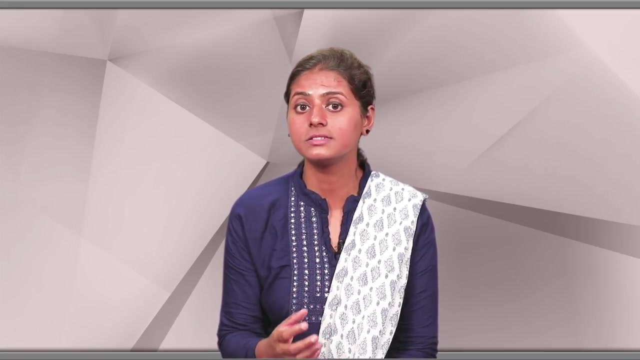 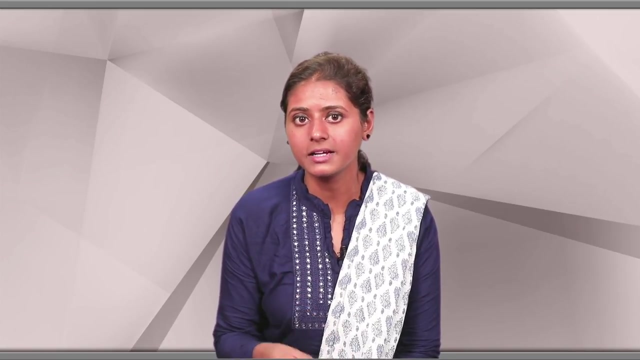 The higher the temperature, the more vapors are released. Mercury vapors are colorless and odorless, Though they are visible in ultraviolet light. mercury is liquid at ordinary temperatures. Mercury is also called quicksilver. It is a heavy, silver, white liquid metal and it is 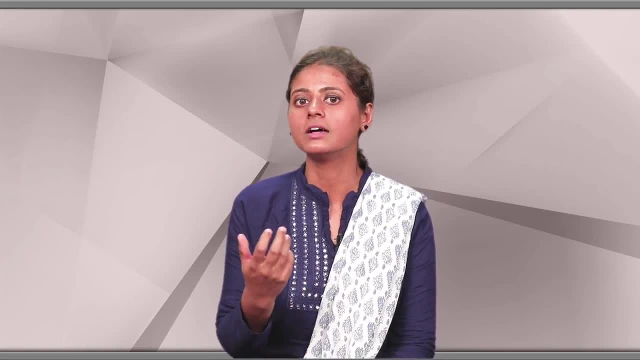 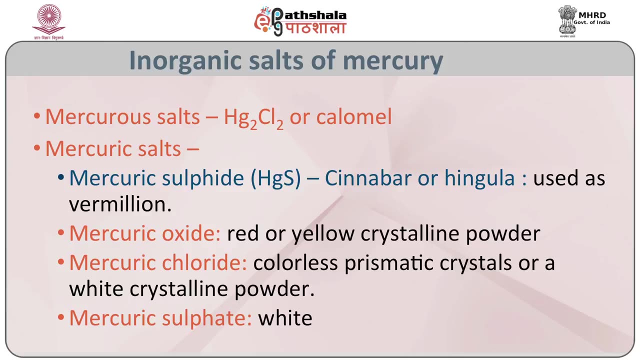 a poor conductor of heat but a good conductor of of electricity, So it can conduct electricity also. The most important and mercury salts are mercury chloride, HGCL 2, which is also known as chlorine. Chlorine is a corrosive or sublimant mercury chloride, HG 2, CL 2, chloramine or mercury fulminate. 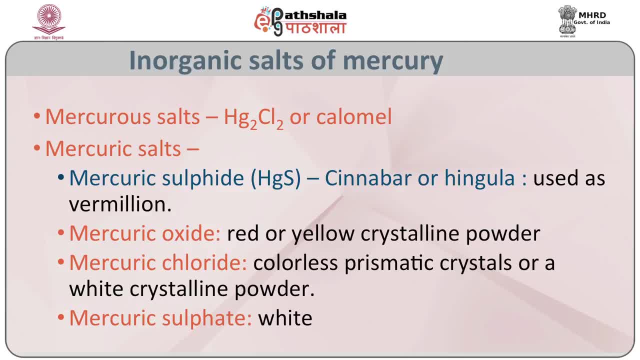 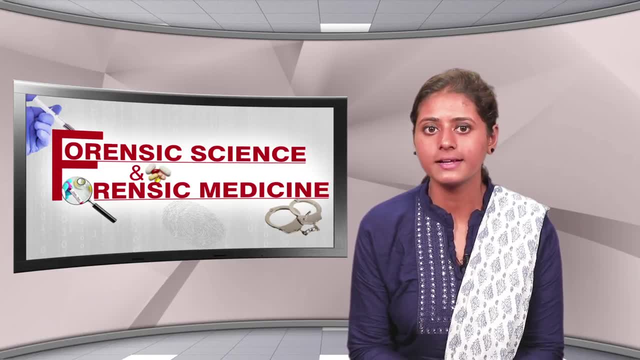 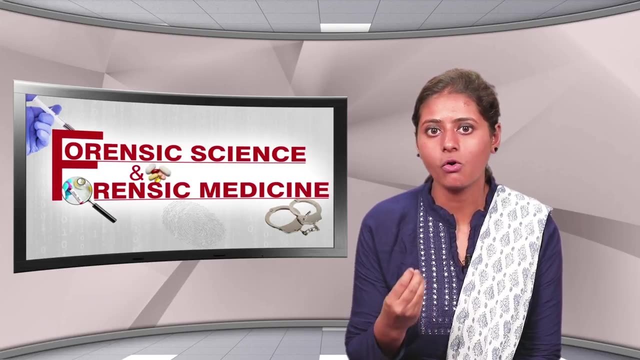 HG ONC 2.. Detonator used in explosives are mercury sulfide, HGS, vermilion or uses of compounds of mercury Inorganic salts, mercurous chloride used as fugitive, or which is known as mercurial ointment, ointment third, or maybe called as ointment fourth. 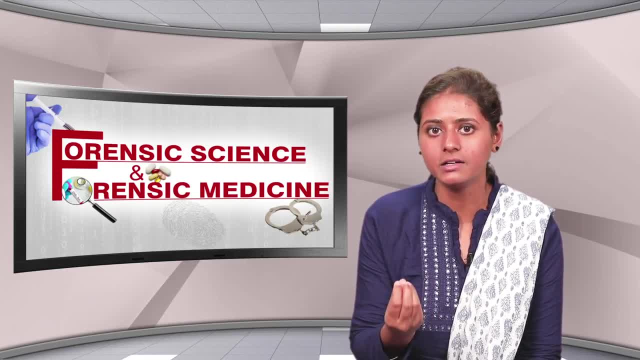 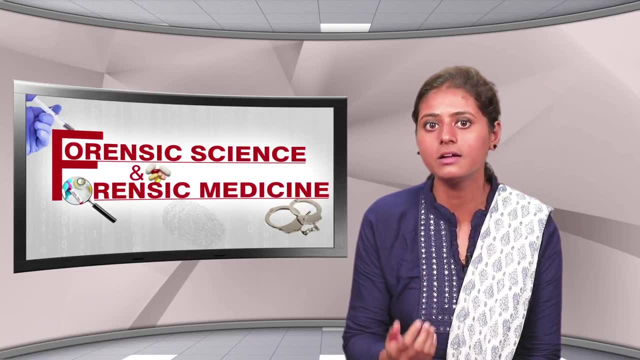 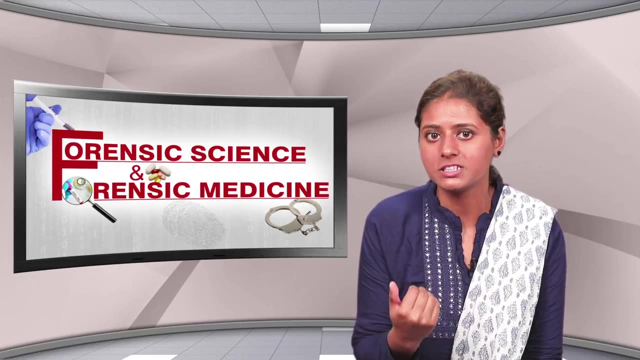 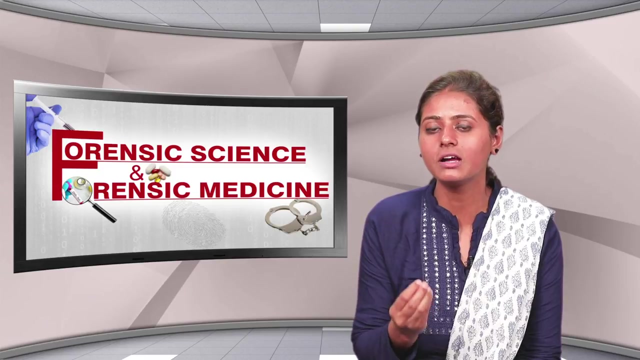 Or fingerprint powders, amalgam, vermilion. second, organic salts are used in manufacture of thermometer, barometer, electrical industry. or, fourth, maybe drug manufacturing or in agriculture as fungicides. Acute poisoning of mercury, which includes, mostly due to corrosive sublimant, mercury chloride. The signs and symptoms starts immediately after. 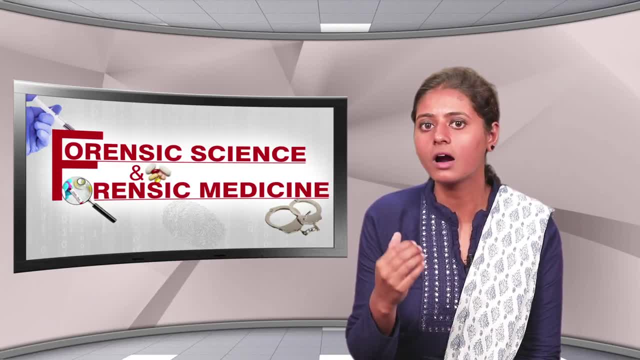 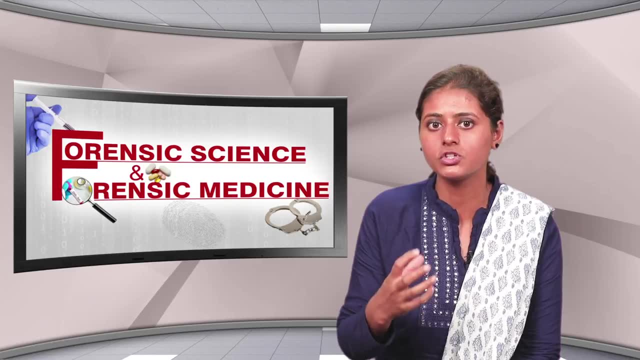 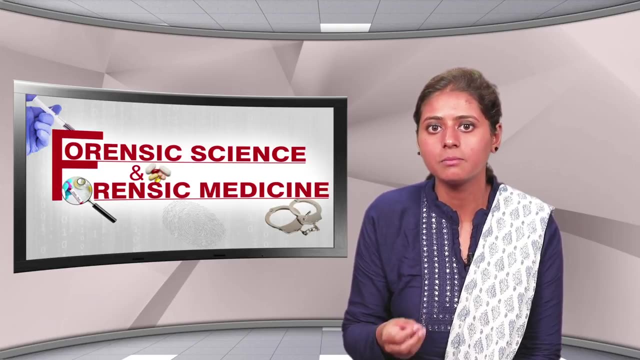 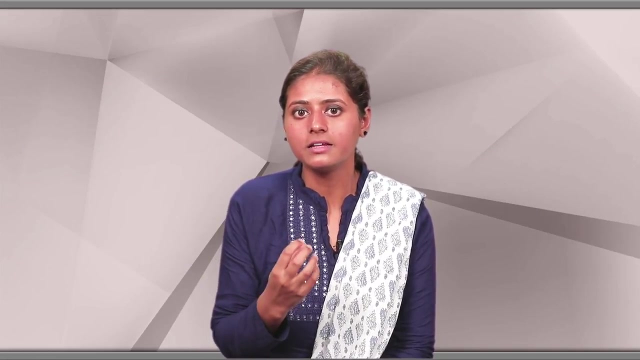 swallowing the poison and rarely delayed for half an hour, which is accurate. metallic taste in mouth, feeling of constriction, of choking sensation or harsh voice, which can be done by mercury, or difficulty in breathing. mouth and tongue corroded and swollen with a grey white coating, Burning pain in mouth, stomach and abdomen. The stools stained with. 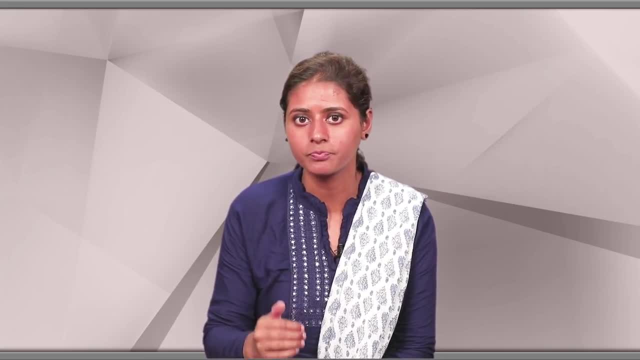 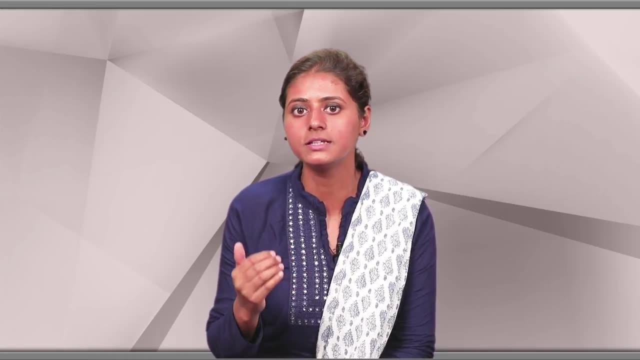 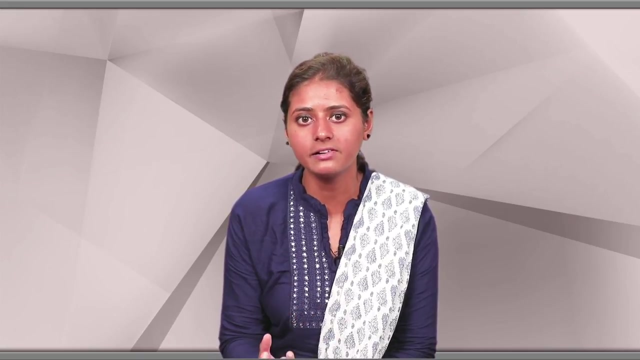 mercury chloride. Urine is suppressed and scanty, which maybe contain blood and albumin, Is accompanied by the necrosis of renal tubules and damage to glomeruli. The pulse is quick, small and irregular. There is circulatory collapse. the thrombocytes and bone marrow 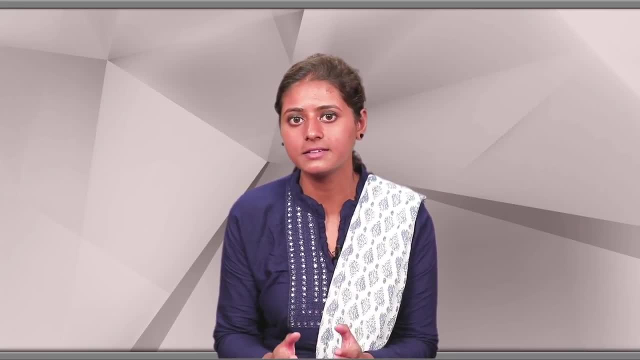 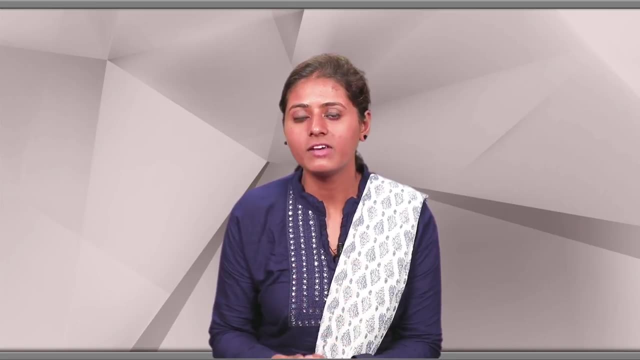 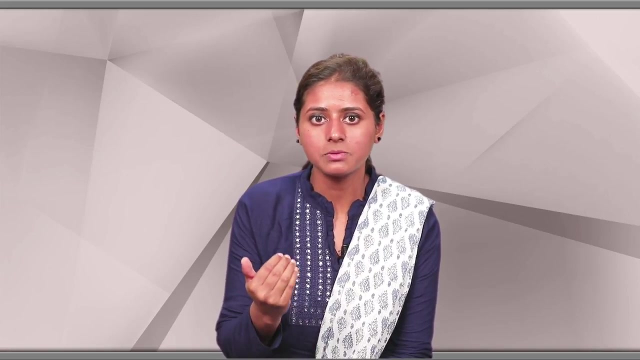 depression. when vapor are inhaled, The following signs and symptoms are produced, which is maybe salivation, Ginger virus, Enzymatitis and loosing of teeth. When injected vesinally it causes dyspnoea, synopsis, hypotension and conversions, or may be death. may. be due to and afaxactor shock or ventricular fibrillation. We will discuss about the fatal dose. The fatal dose is about 15 gram to 2 gram is the smallest recorded dose. The fatal period, which include is 2-3-0-6- pages in cycle period. Body. 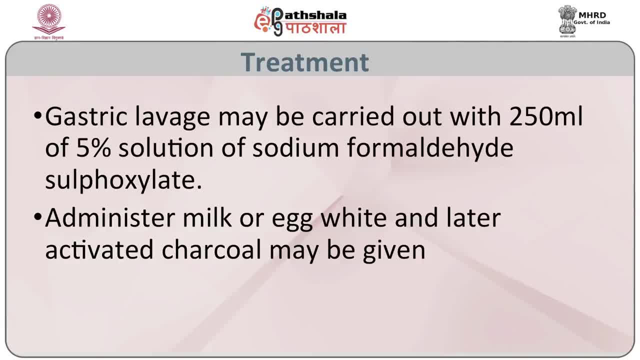 include is about 3 to 5 days, and the treatment of the mercury is gastric lavage with a sodium. formaldehyde sulfoxylate or Baal is a chelator of choice, or pencil amine or sulfoxylate, which is about 10 gram in 100 to 200 cc of distilled water by slow. that is why intravenous injection. 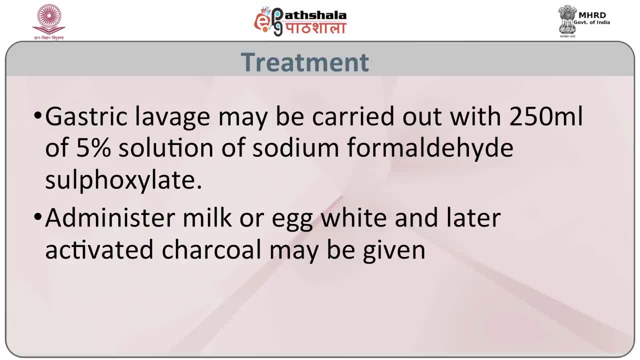 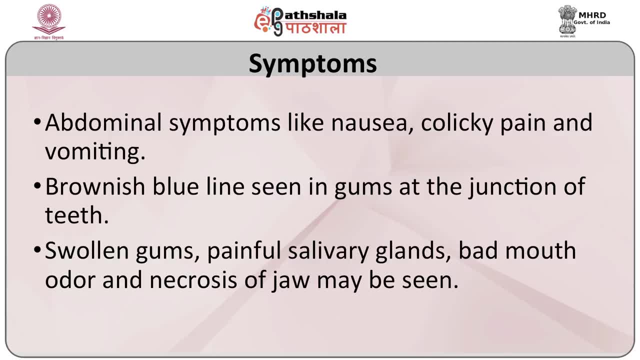 in repeated doses at every 4 to 5 hours act as an antidote. the chronic mercury poisoning: we will discuss our chronic mercury poisoning poisoning. the symptoms are salivation, blue line on gums, sore mouth, the throat line, tremors of their tongue, hands and arms. anemia may be also be there, shaking. 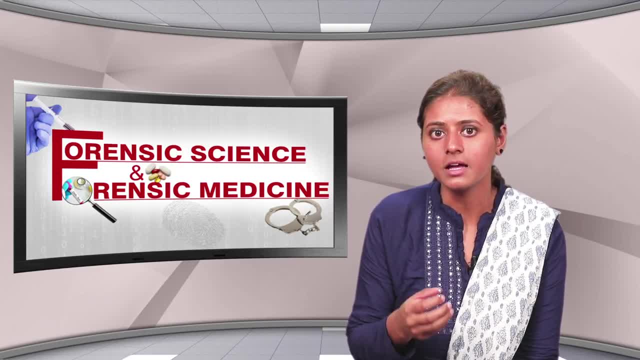 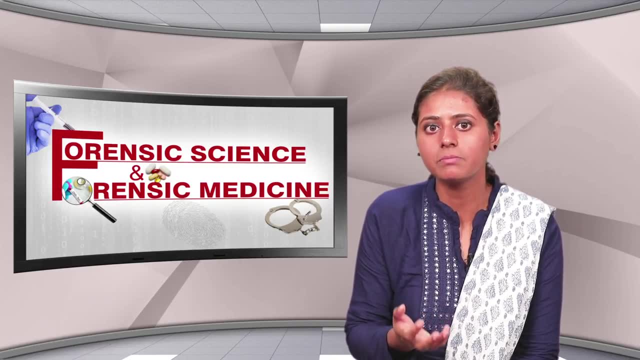 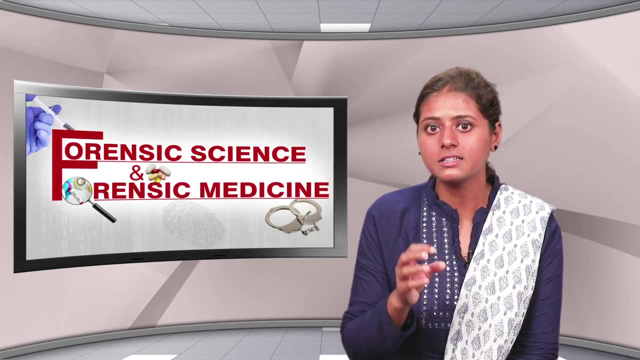 palsy is associated with the edgy poisoning. mercury tremors are also called as hater's symptoms, shakes or mercury racism is seen in person working in mirror. manufacturing informs where Merrick is used in it's isma is a characterized by the shyness or remedy, or irritability loss. 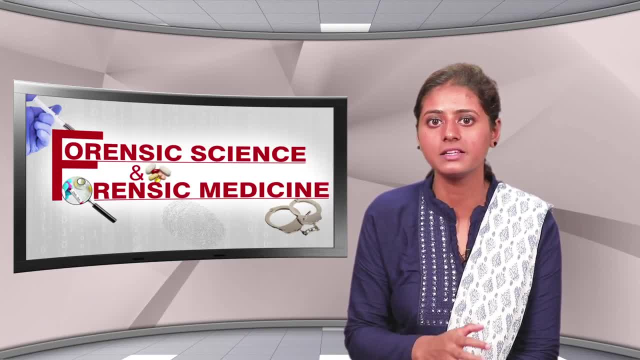 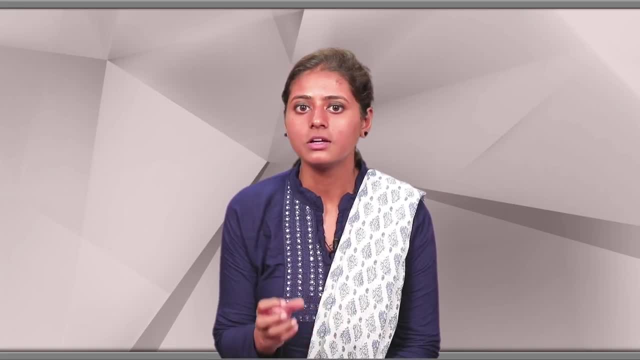 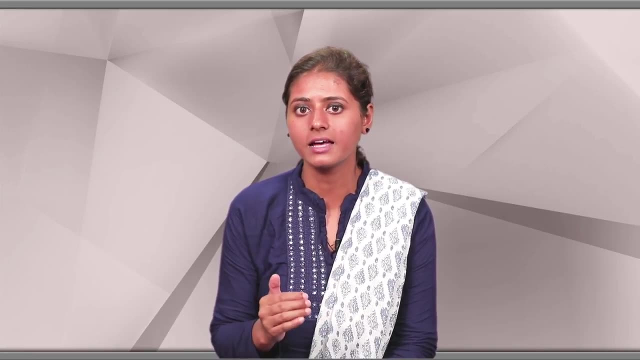 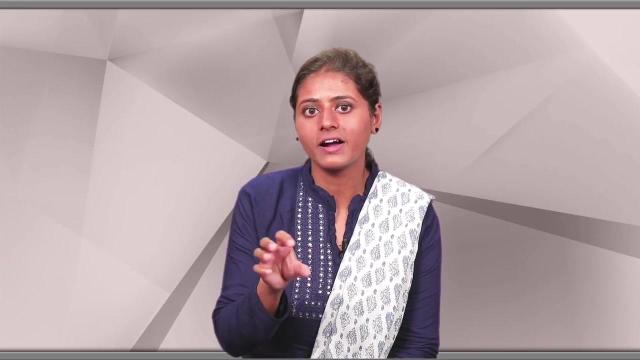 of confidence, mental depression, loss of memory and insomnia. mercury lentis is a peculiar eye change due to brownish deposit of mercury though the chronia of the entire length of the capsule. it is bilateral and has no effect on visual equality. Autopsy which, based on the mercury, are findings, if it taken in concentrated form, appearance. 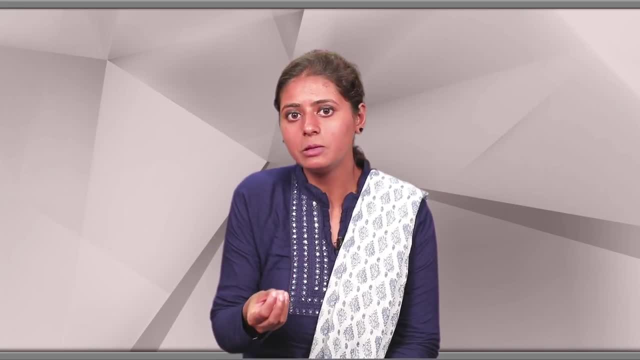 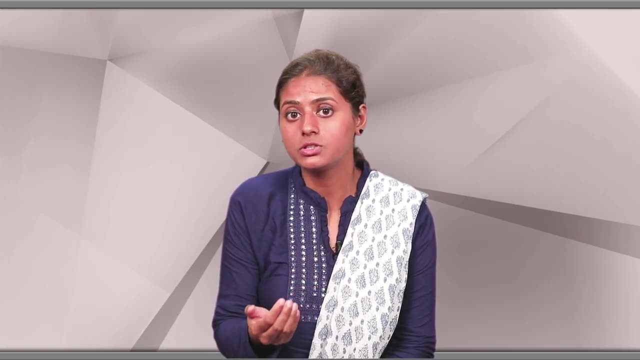 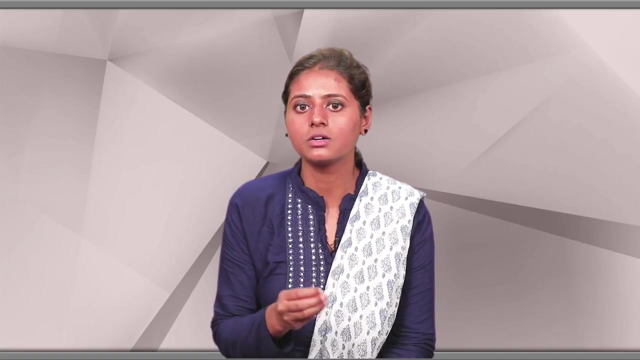 may be similar to corrosive poisoning and it will be present. The signs of irritation of mucosa, membrane of line, lips, mouth, pharynx and oesophagus will be grayish, white and stomach contents are coagulated albuminous with mucus and blood. 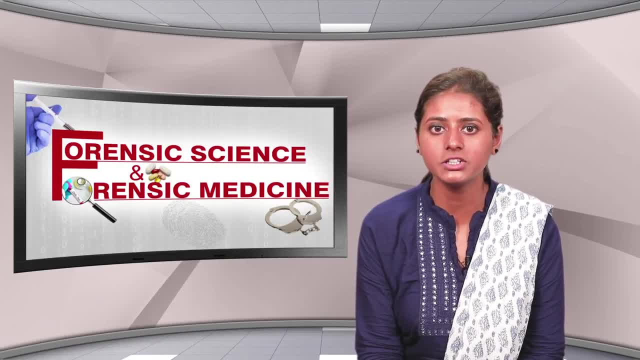 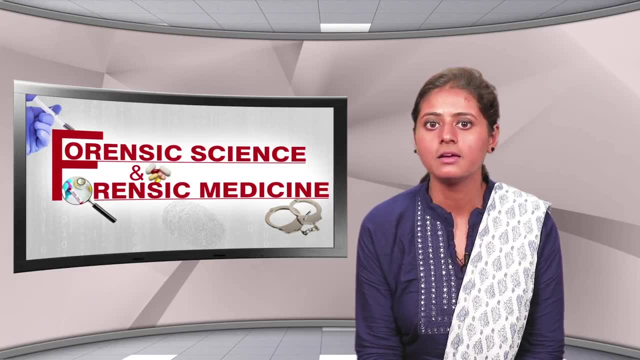 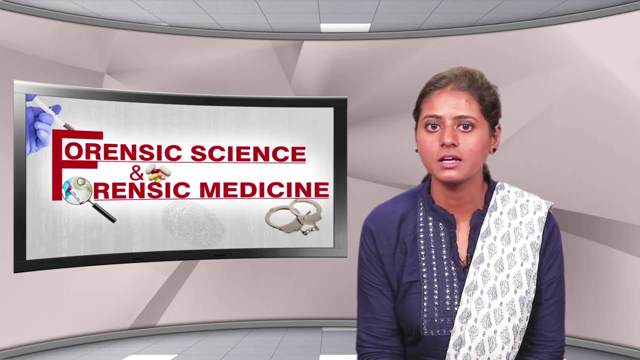 Mucus membrane is eroded, inflamed and covered with grayish or black deposit, The deposits of mercury and compound. softening of the walls is so great care must be taken during post mortem examination to remove it. perforations are rare, cecum, colon and rectum. 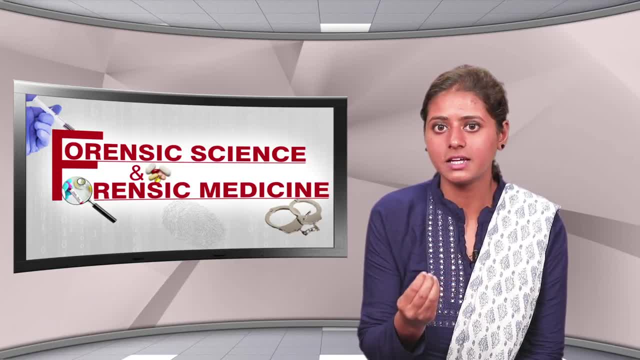 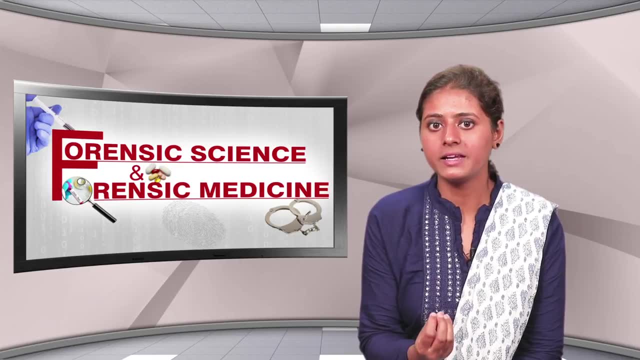 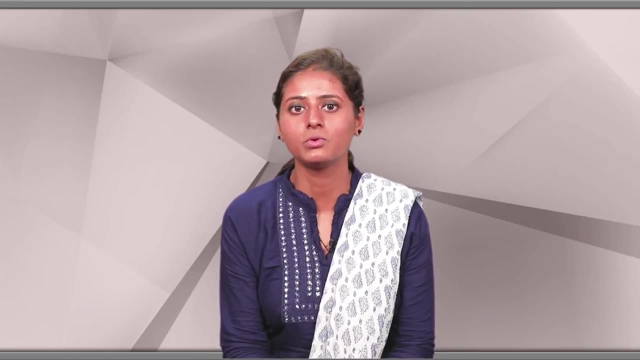 are inflamed, ulcerated and gingivism is alive, for sometimes liver is congested, with cloudy swelling. spleen is congested, kidney are may be congested or there is a necrosis of tubules and deposition of lines. heart shows fatty changes. post mortem lessons are: 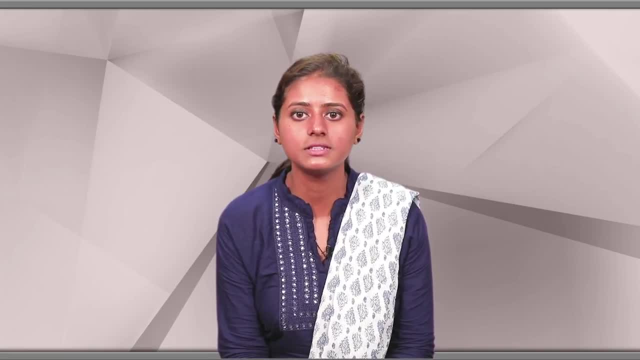 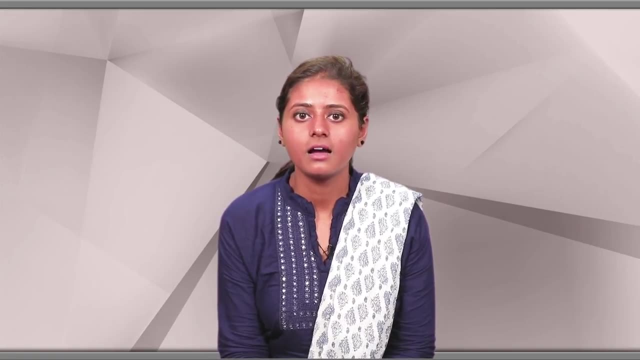 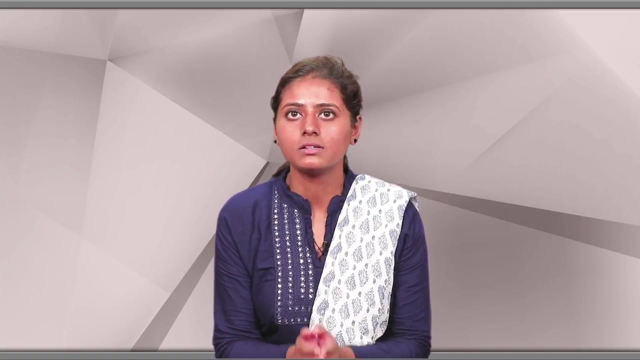 found in the alimentary canal, even when applied on the skin or absorbed from the vagina or uterus. That's all for the lesson. we learn about the heavy metal poisoning and we learn about arsenic, mercury, so these are very dangerous and we should not use lead as a eyeliner or 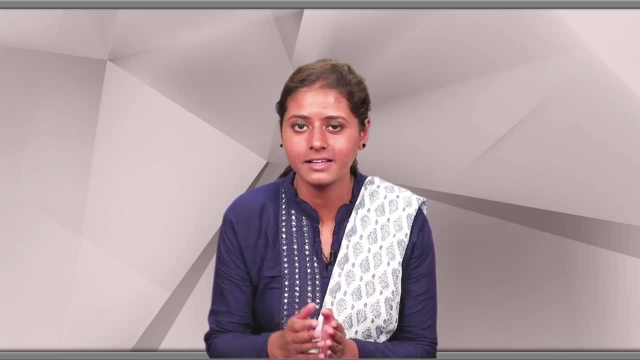 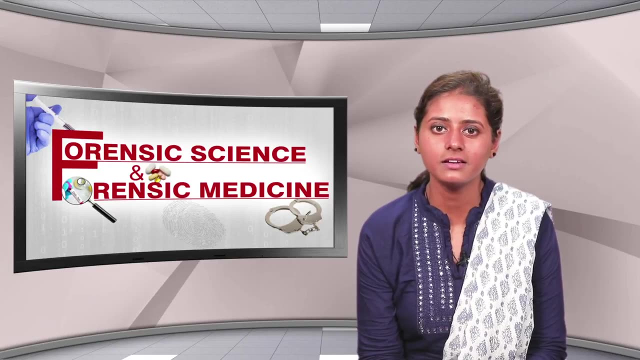 may be in lipstick. they are lead using and arsenic. our products were there, So thank you for the today's discussion on heavy metals poisoning. Thank you. Subtitles by the Amaraorg community.